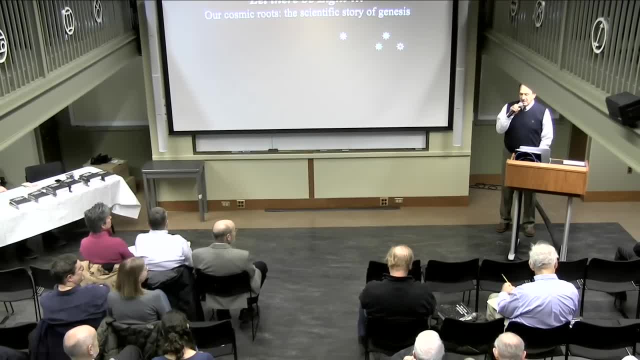 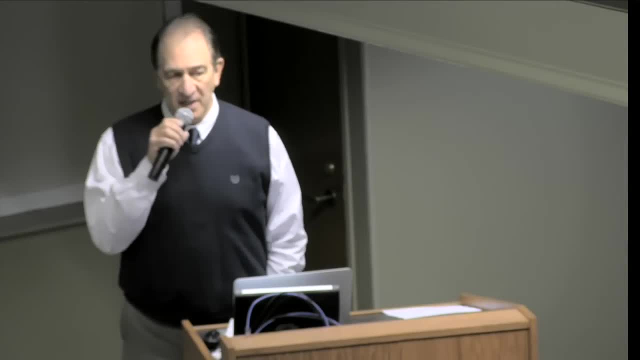 and say: explain to me everything I need to know about string theory in the next 15 minutes. It's going to take 20 minutes, But when you leave, your brain will be larger than it was when you stepped in through the door. 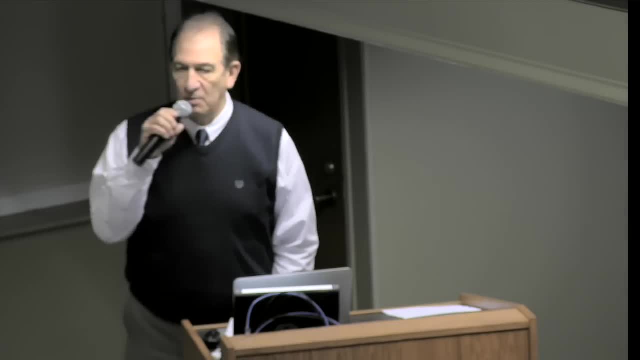 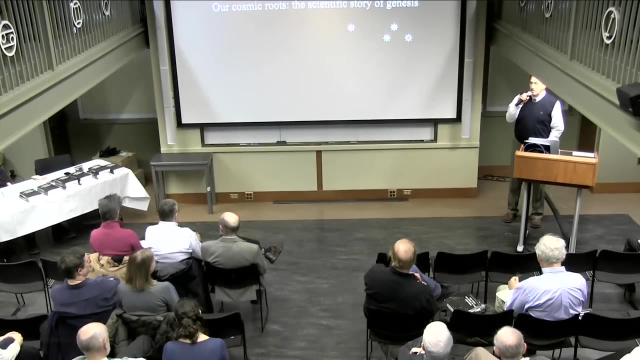 Working in my position, I realized that so many of us use telescopes and instruments to cruise the universe to unravel the clockwork of the mechanisms of how this universe around us works. But there is a very special group. we've given them the name cosmologists. 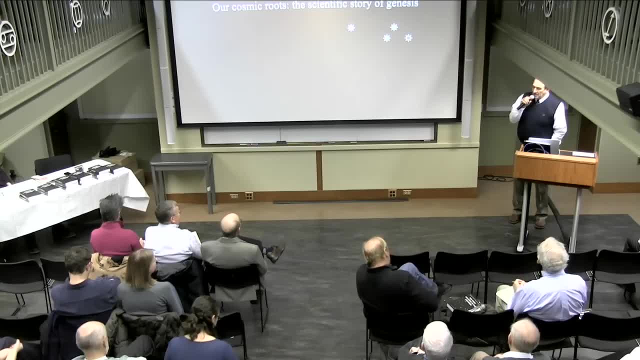 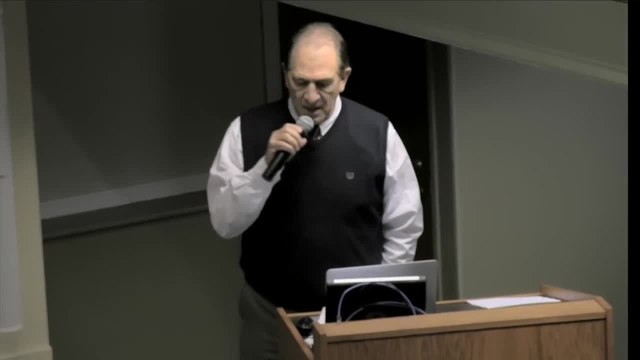 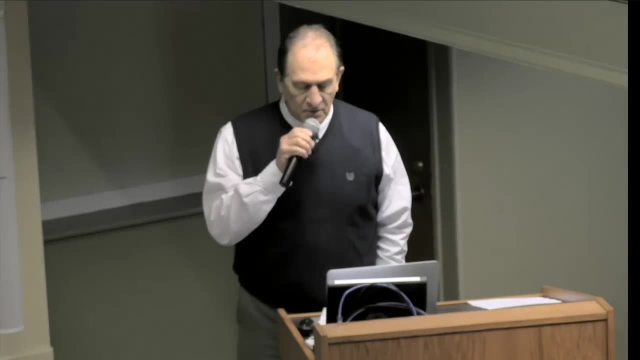 that cruise the universe. sometimes in their minds They approach it- life here on Earth, the creation of the universe- very differently To them. the music of the spheres plays out in the key of mathematics. When I do general talks and I get to tour around the world, 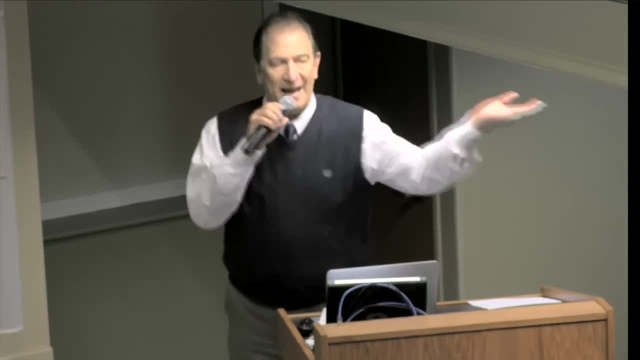 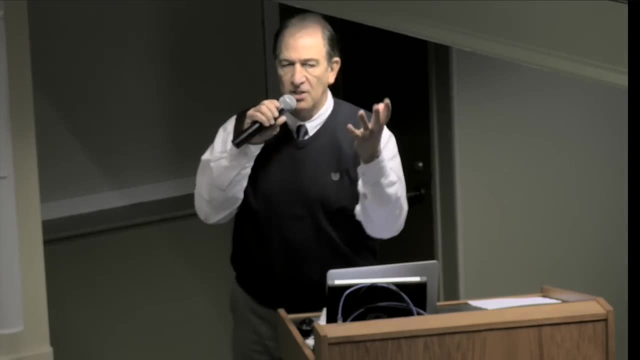 people are so interested in exoplanets, they're interested in black holes, they're interested in supernovae, but something happens when the subject turns to dark energy, dark matter, the Big Bang, the beginning of the universe, string theory. 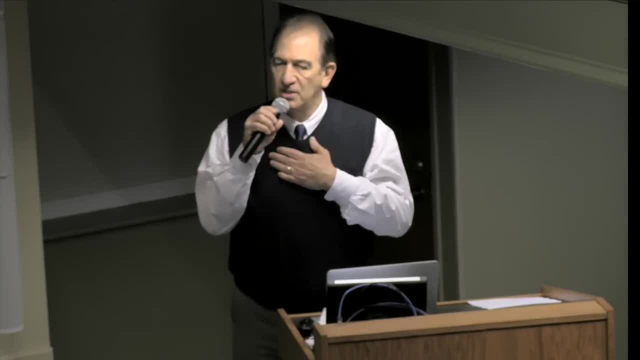 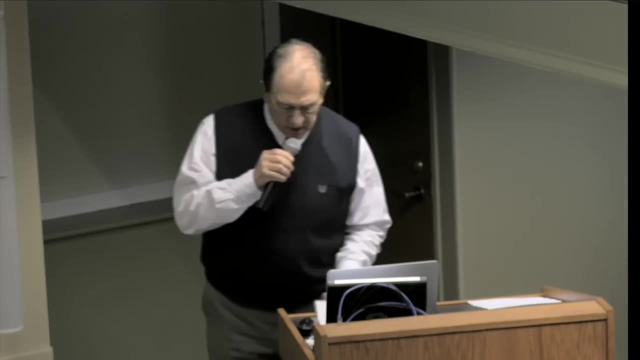 For some reason, it touches the heart and the soul in a very different area than some of the other parts of the universe that we study do, And I don't quite sometimes understand this. In 2008,, Avi wrote his first book. 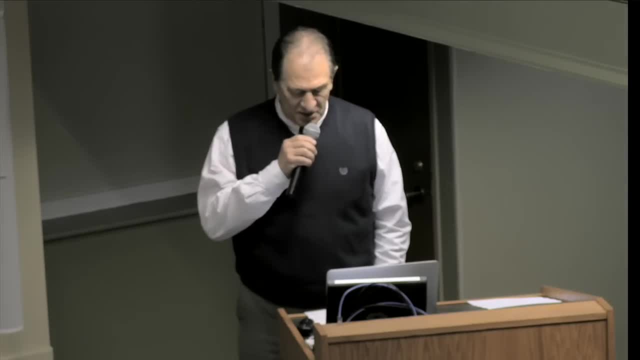 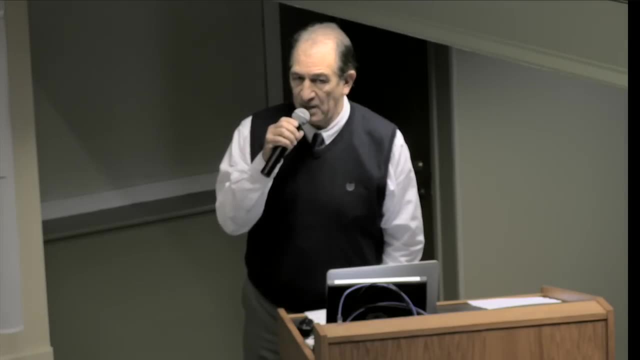 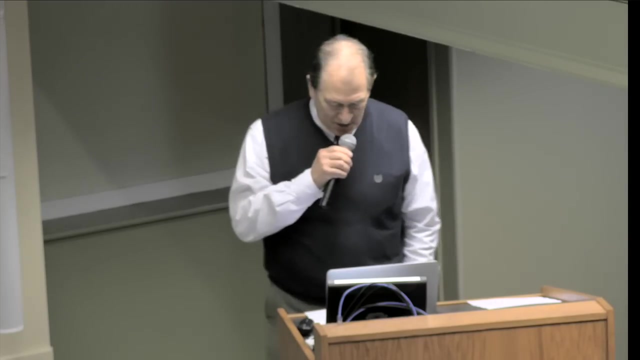 First Light in the Universe In 2010,. he wrote: How Did the First Stars and Galaxies Form, which just won the Best Science Writing Award at the American Astronomical Society meeting in Long Beach this year, Congratulations. And in 2012,. 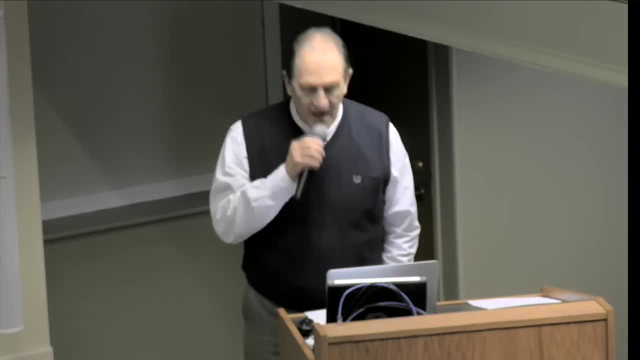 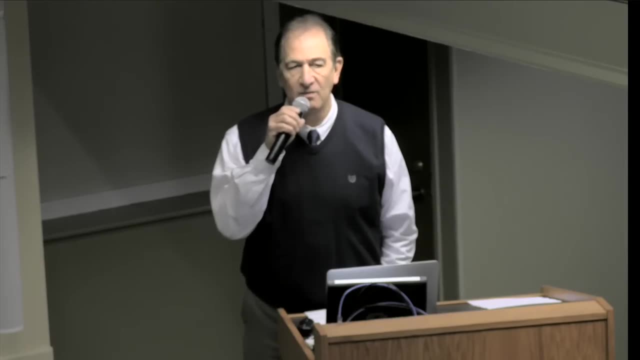 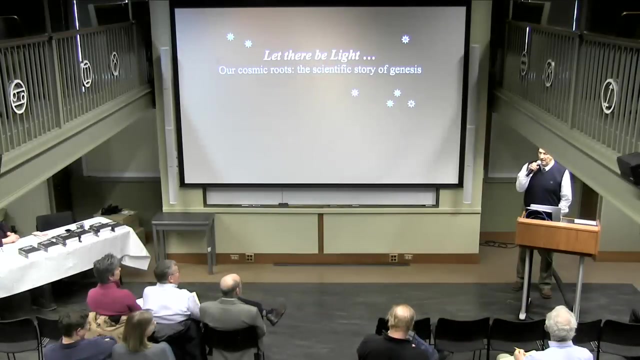 The First Galaxies in the Universe. I asked a graduate student because I had not had time to read the book, how was it? And she said it was wonderful. And I said to her, in so many words, how can you describe this book to me? 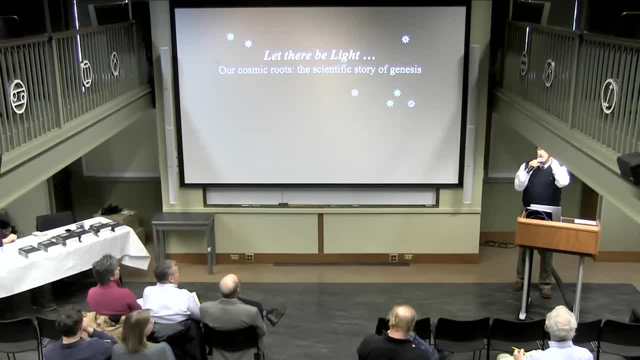 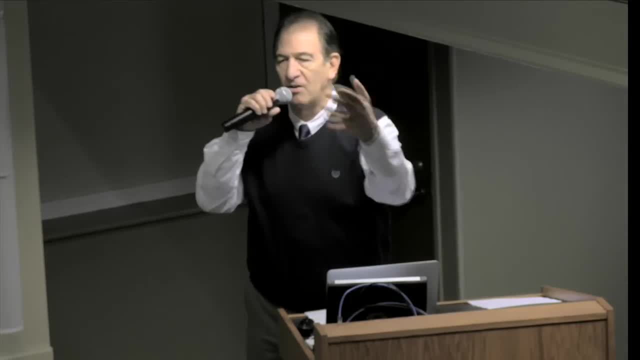 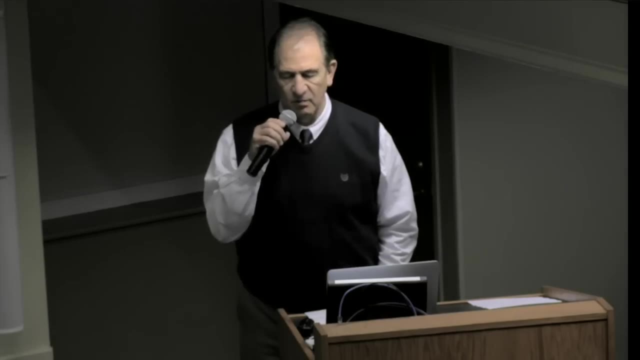 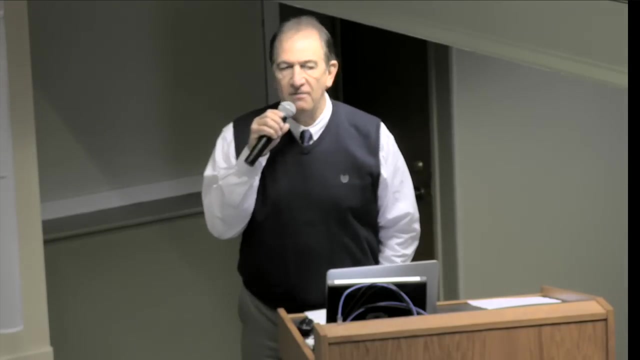 And she said: well, think of it as a family album, with the first baby pictures of the universe spread on all the different pages. Writing a book: what an adventure. You give up part of your life, you change. You're thinking about it every moment of the day and night. 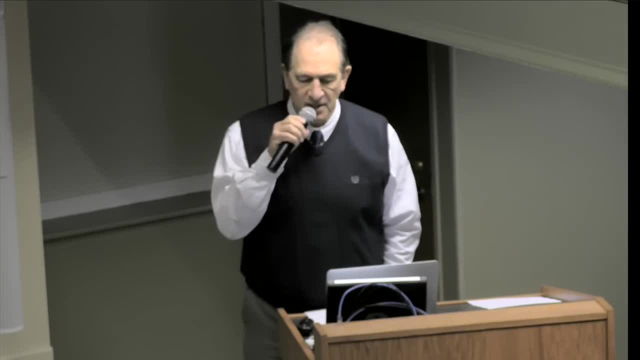 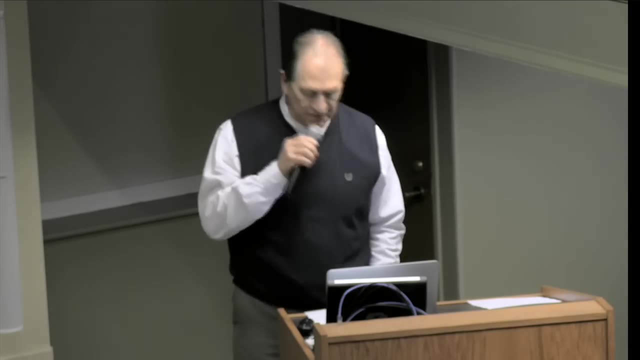 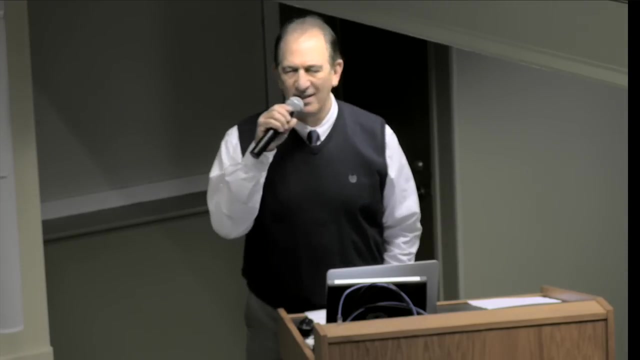 You're changing, you're wondering, you're directing, you're moving things here, you're moving things out. It's a labor of love, a dedication, of frustration, of perseverance, of sacrifice. Did I mention dedication? And when it's finally done, 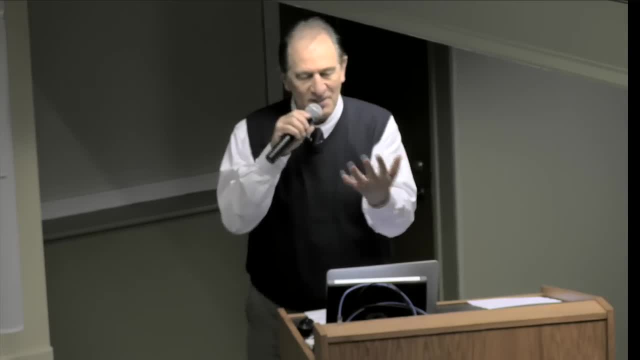 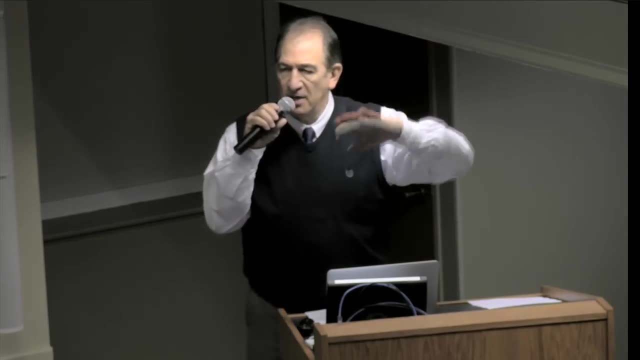 there it is. You can hold it in your hands and feel it, and look at it and live with it. When I go back to my office, there are books on my shelves that are old friends to me. They're written by Owen Gingrich. 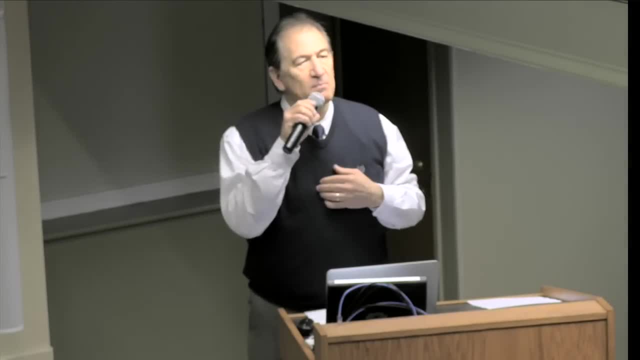 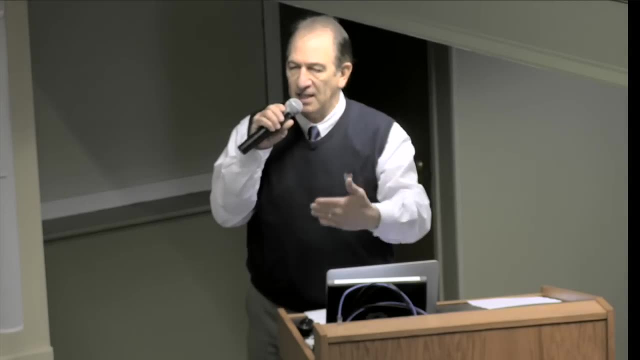 They're written by Bob Kirshner, They're written by Bart and Priscilla Bach, They're written by Harlow Shapley. And these texts live on and on in our lives. And now I'm about to add one more book to my shelf. 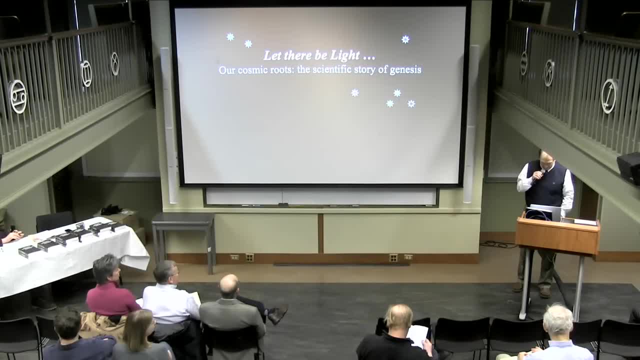 The First Galaxies in the Universe. Now I've noticed a pattern here. First book came out in 2008.. The next book 2010.. This book 2012.. I hope there's something coming out in 2014.. 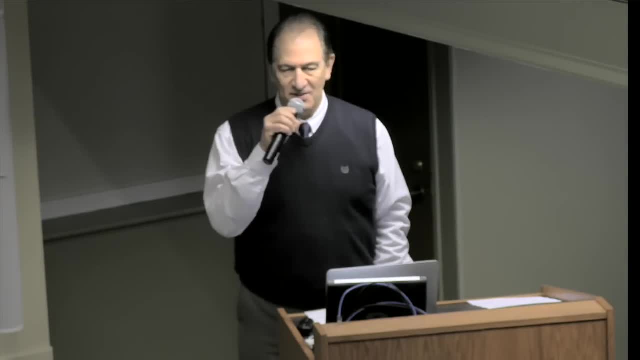 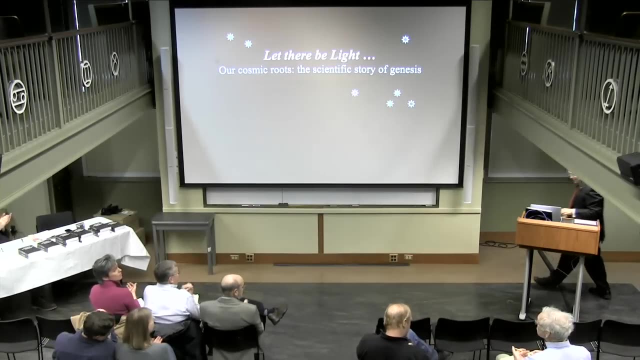 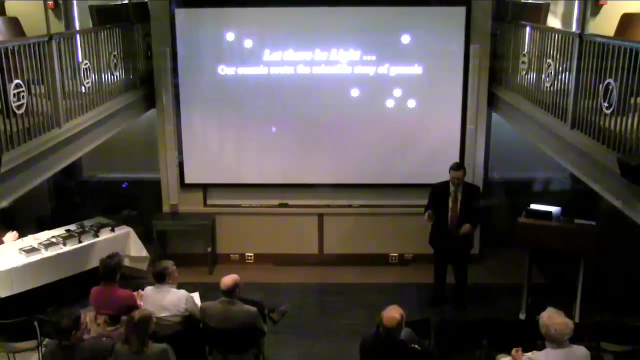 So it is my great pleasure to introduce to you Avi Loeb. Thank you very much, Dave. That was very kind, And after such an introduction I should say that if my father was sitting here he would have been impressed. 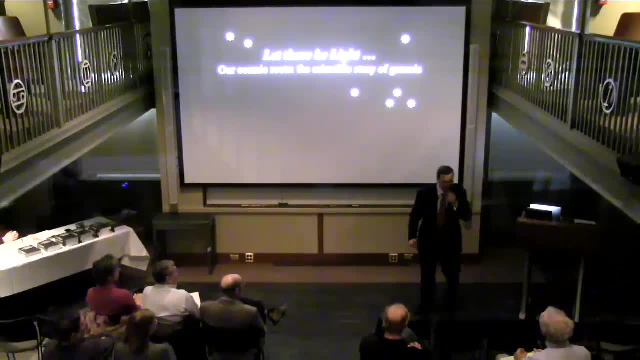 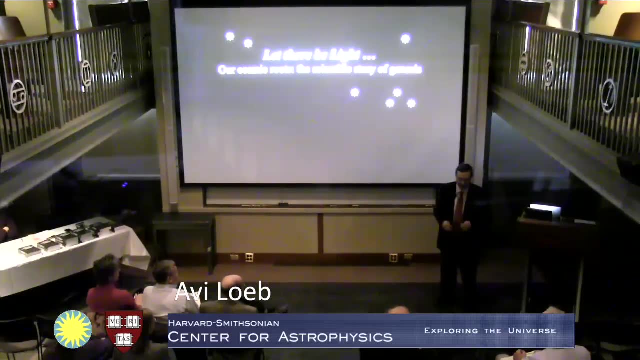 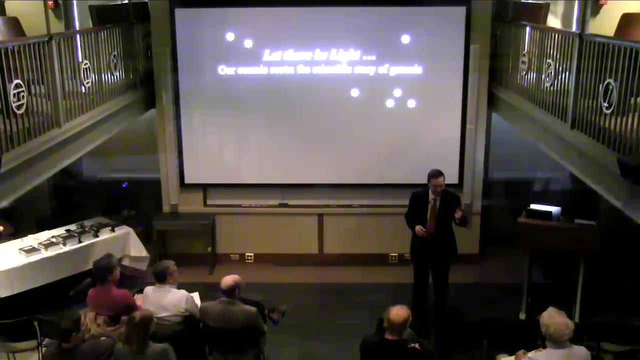 If my mother was sitting here she would have believed it. And speaking about family, I should also mention that I mean I obviously thank my parents for giving me life, But I especially thank the three women in my life, one of whom is sitting in the back there. 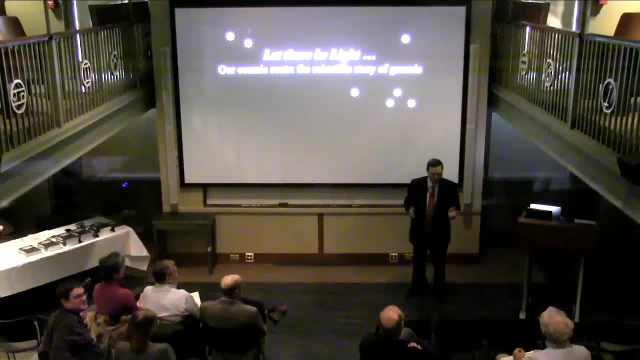 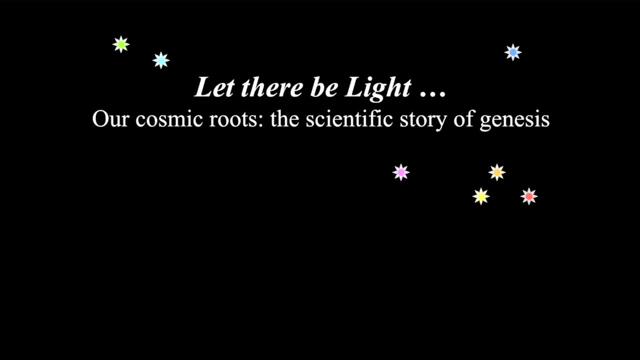 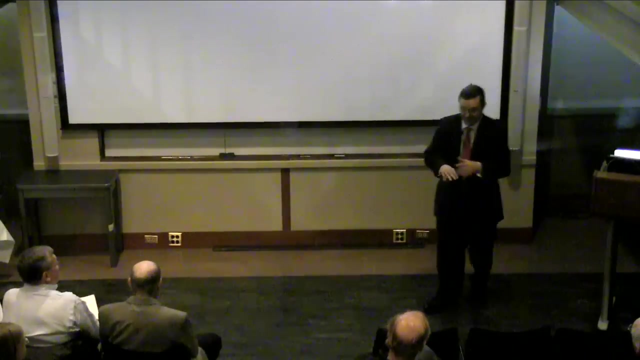 Ofrit and my two daughters for making it worthwhile. And just an introductory comment: If we think about our life as a play, it's obvious that our sin occurs at a relatively late act. in this play We live, we stand on the surface of a. 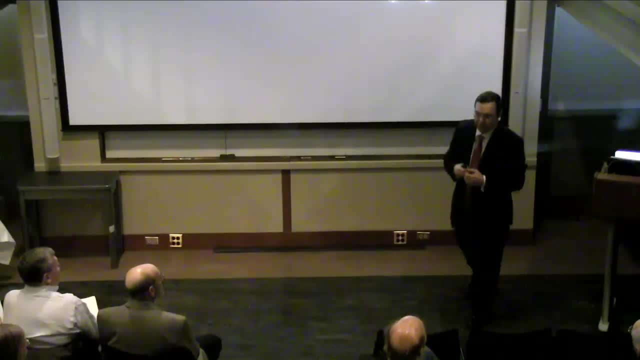 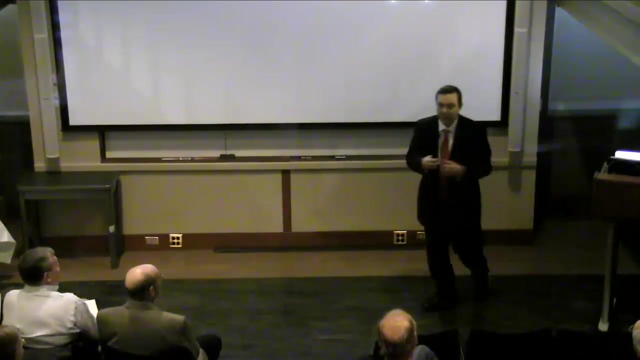 piece of rock that we call the earth, which orbits a star that we call our sun. that is one out of almost a trillion stars in our galaxy that we call the Milky Way Galaxy, which is one out of a trillion galaxies that we can see out there. 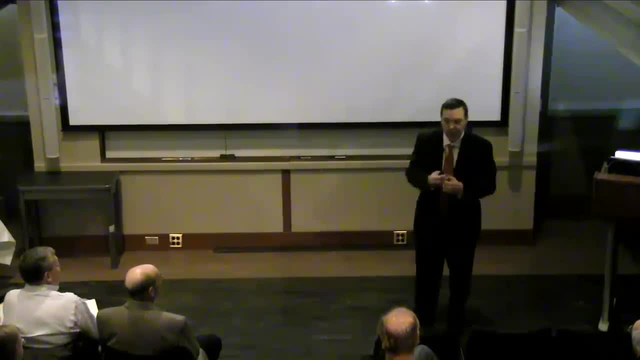 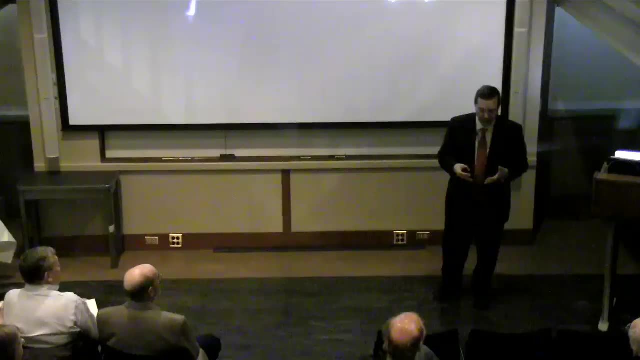 that are running away from each other in the cosmic expansion. And if we just ask what happened before then, What? if you want to understand how we came into this scene that we are in right now, we would like to go back in time. 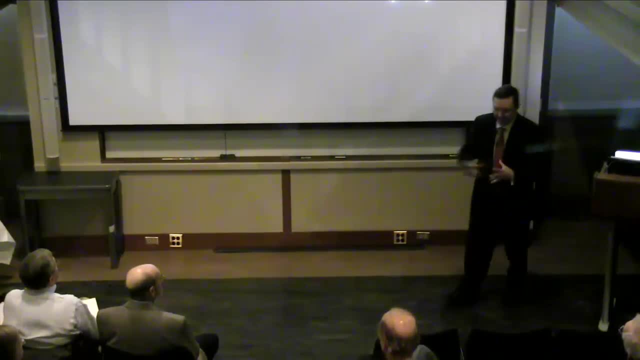 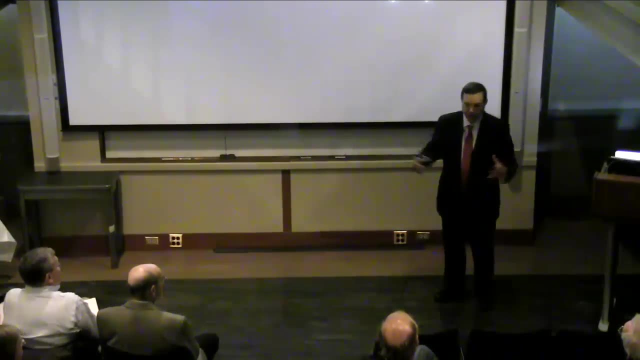 And if you reverse this expansion and go back in time, it's clear that we are dealing with a contracting universe, and the density of matter would increase indefinitely, eventually reaching infinity, at a point in time that we call the Big Bang. That's when the expansion started. 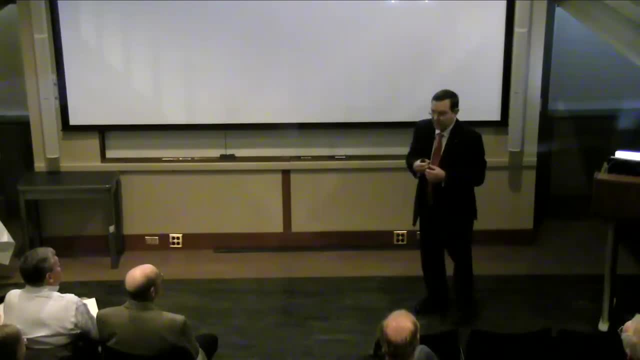 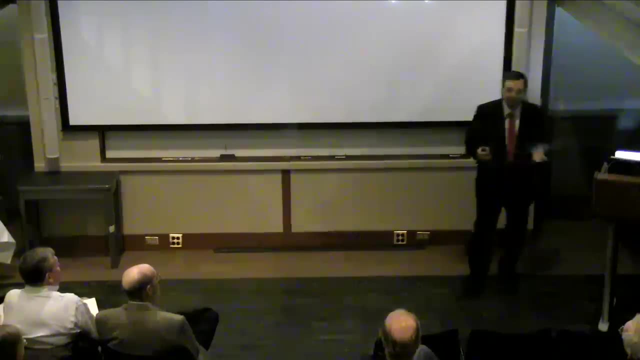 And as you go back in time, there was obviously a time when a time when the density of matter was higher than the density of the Milky Way Galaxy. And, if you go farther back in time, there was a time when the density was higher than the density of the sun. 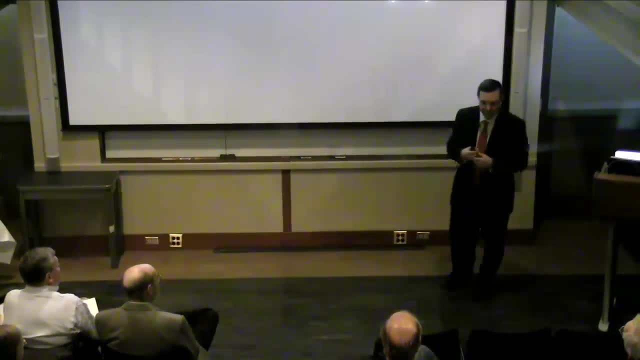 So, obviously, the sun or the Milky Way Galaxy did not exist forever. they were made at some point in the evolution of the universe, And what this book that I described is trying to lay out is the physical processes that may have led to the formation of the first stars and galaxies. 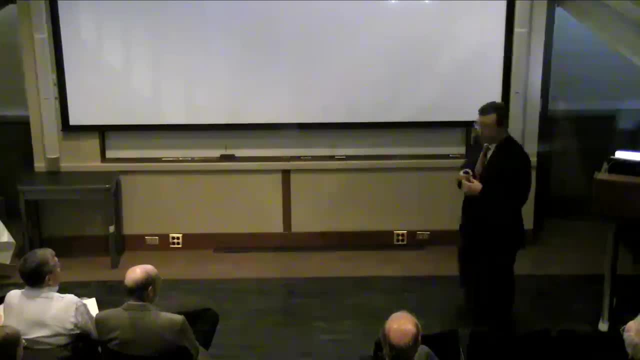 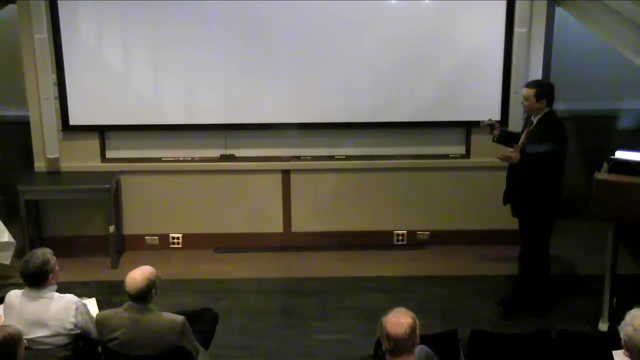 And these represent our cosmic roots. It's basically the scientific story of Genesis, how we came into existence, And, as you well know, there are earlier versions of this story. you can find them in the first chapter of the Bible And, of course, these ancient stories. 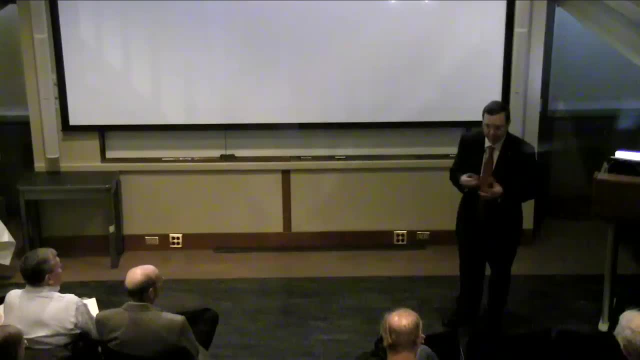 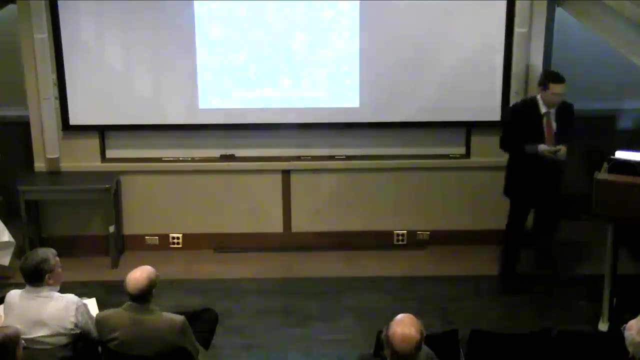 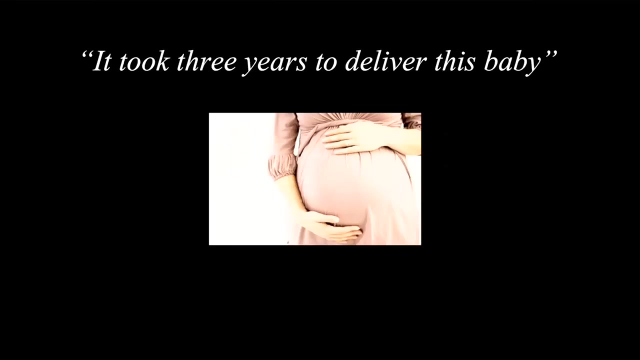 either in religious or philosophical texts need to be revised. It's about time that they should be updated, given all the available information. So that's the cover of my book. It's very detailed, about 540 pages, And it took three years to deliver this baby. 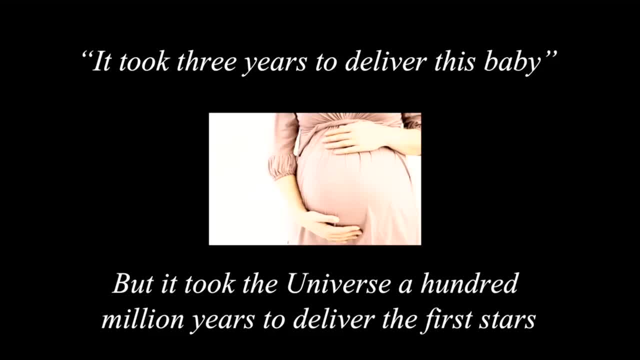 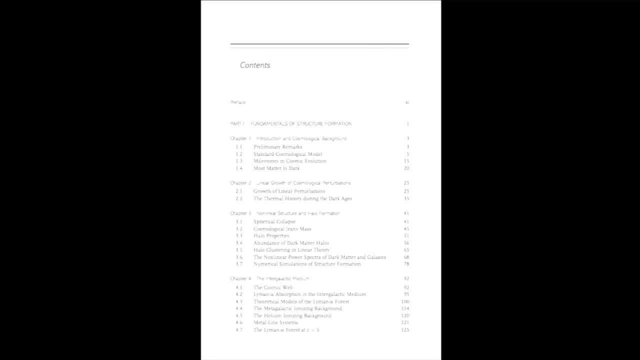 But I should not complain, because it took the universe a hundred million years to deliver the first stars as I described, And the book was written with Steve Forlanetto, who used to be my student here in the astronomy department. He's now a professor at UCLA. 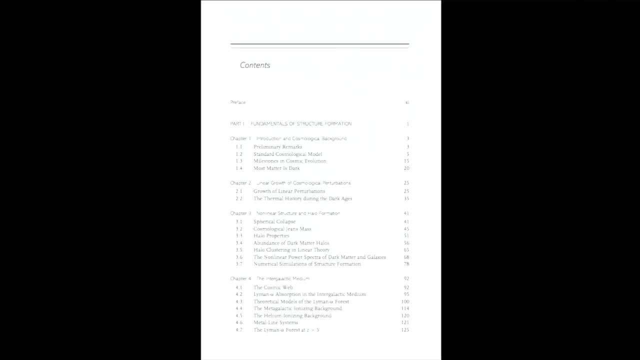 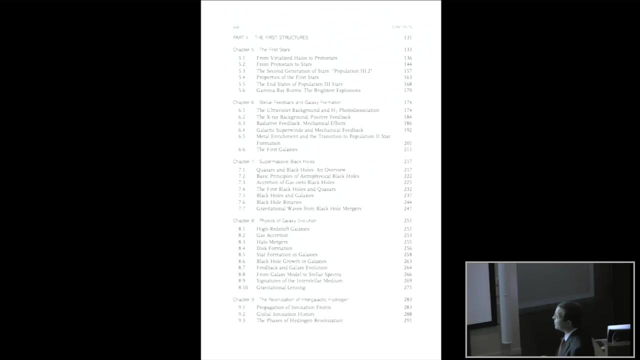 And the book is divided into three parts. In the first one we described the fundamentals of structure formation, how structure forms in the universe, the expanding universe, including both galaxies and the medium in between galaxies, the intergalactic medium. Then we discussed the details of those structures. 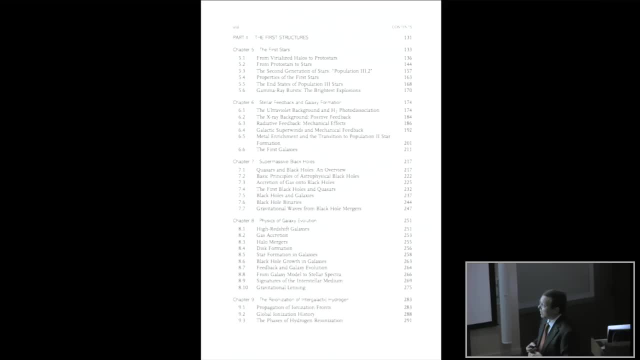 in particular, how did the first stars form, which feedback effects they had on their environment, the formation of supermassive black holes and the evolution of galaxies and, eventually, the effect that these galaxies had on the intergalactic medium in between them. 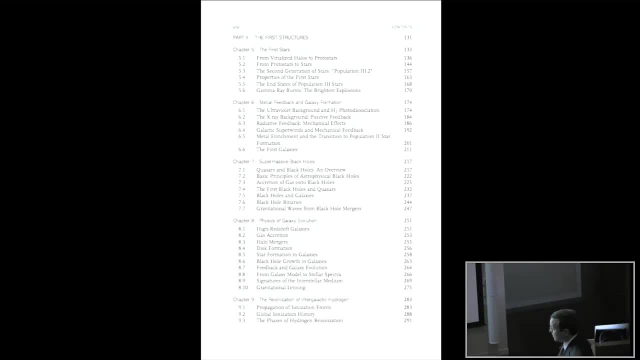 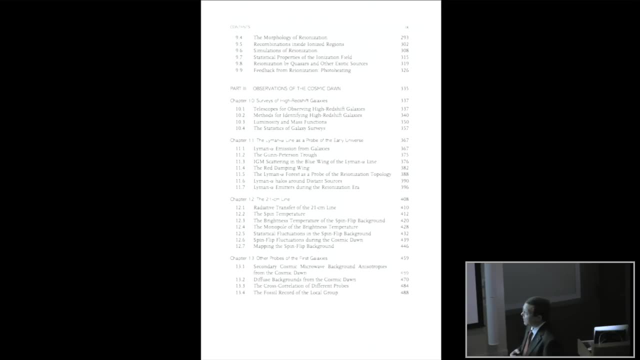 In particular, they ionized, they broke the hydrogen atoms into their constituents, electrons and protons. And finally, the most important part is dealing with future observations: current and future observations of the cosmic dome, And that includes surveys of galaxies and probing the intergalactic medium. 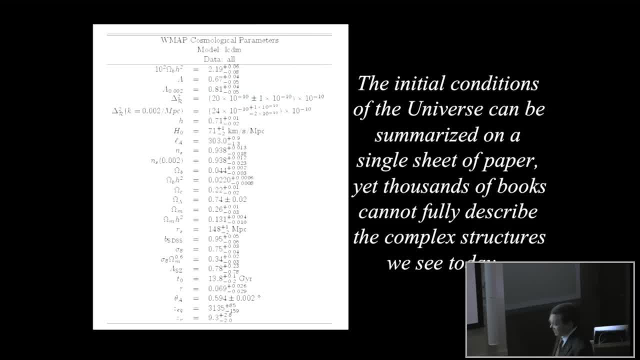 in different ways. So let me give you a few of the highlights of the book of this field. The initial conditions of the universe can be summarized on a single sheet of paper, And we have that sheet of paper. We didn't have it a decade ago. 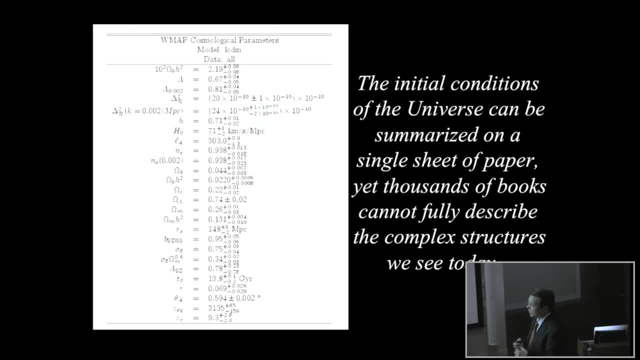 but now we have these numbers, a set of numbers that are known to a very high precision, that can be summarized on a single page. But if we look at the conditions here on Earth, even thousands of books in libraries cannot fully describe them. Just selecting a single topic like politics. 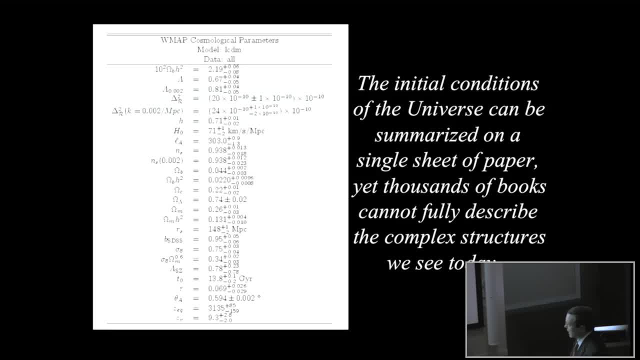 you cannot really fully describe it in thousands of books And somehow the results of the elections, for example, were encoded in these simple initial conditions. You can fit these initial conditions into a computer simulation. run the computer simulation and you will find. 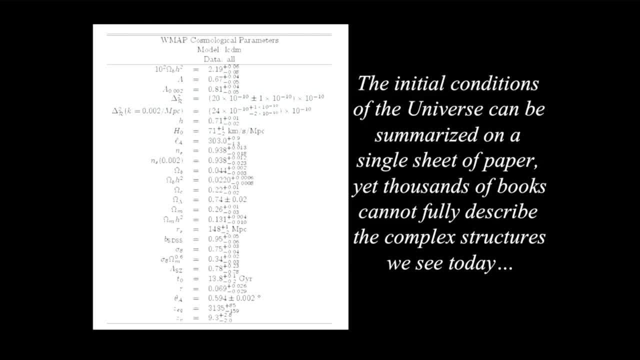 the results of the election. And an interesting question is how come you can start from a very simple initial state in the universe and end up with so much complexity? And the answer to that is gravity. Gravity draws matter together and makes the universe very complex. 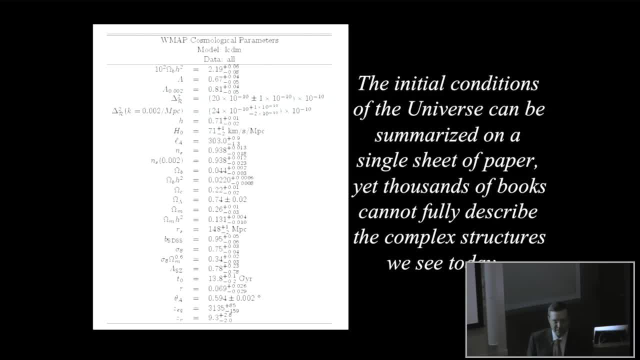 In the early days of cosmology, it was thought that the early state of the universe is thought to be simple, simply because we don't have data. So people thought: well, whenever you don't have enough information, you think that things are simple. 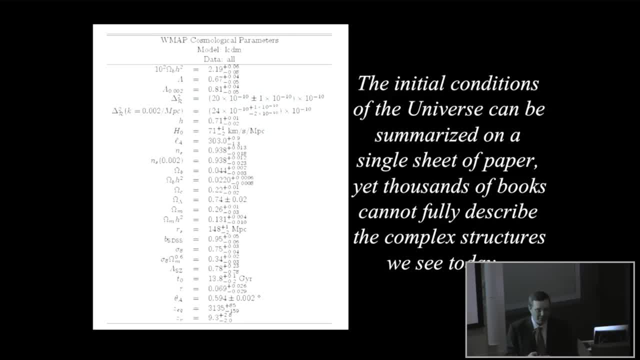 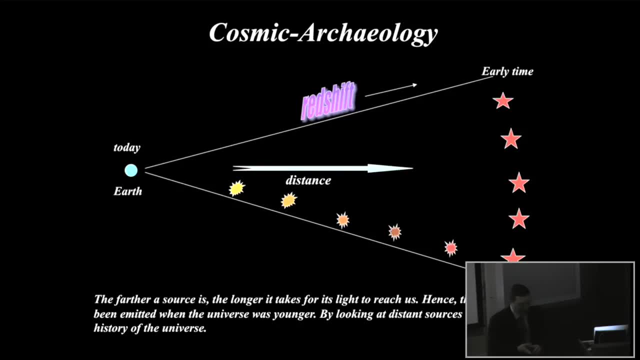 But that turned out to be wrong, because now we have a lot of data from many different probes and it does indicate that the universe started simple. Now, the reason we can explore the past is because light propagates at a finite speed. So when we look at a distant source, 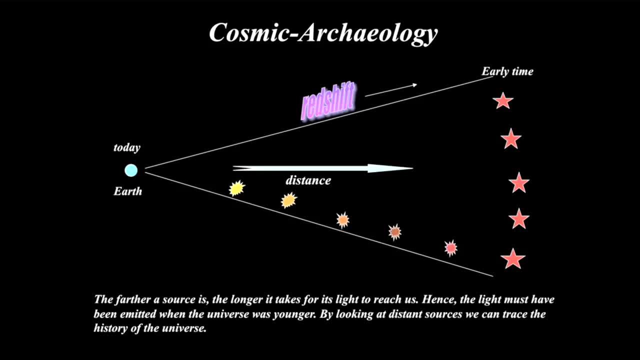 we are seeing how the source looked like at an earlier time, so that the light from that source would reach us today, And so the deeper we look into the universe, the earlier is the time that we are looking at, And it's sort of similar. 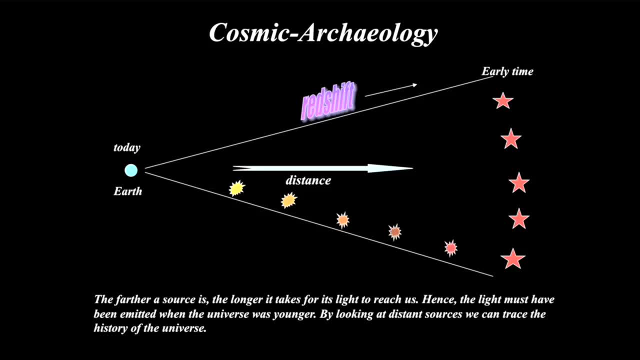 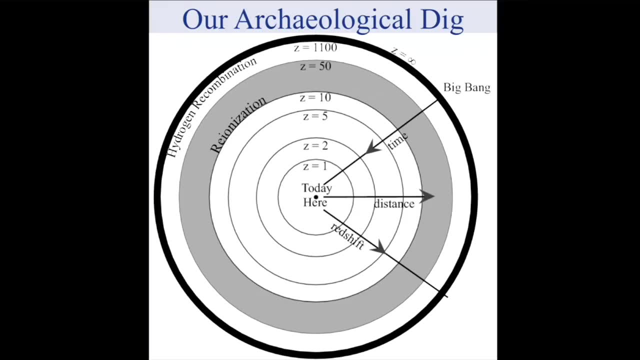 to an archaeological dig where the deeper you dig, the more ancient is the layer that you uncover. And this is our archaeological dig. That's what cosmology is all about. We have an archaeological dig. We're situated in the middle of that. In fact it would look very similar if you were to go elsewhere in the universe On very large scales. the universe started from very similar initial conditions, So it doesn't look very different from other vantage points And when we look out from our point. 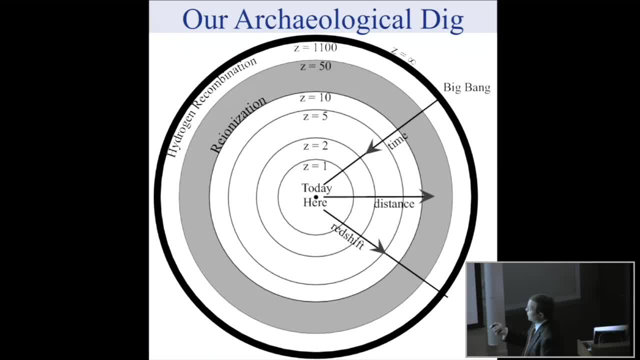 we are going back in time And, of course, the earliest we can see is the point of the Big Bang. So there is a spherical surface around us that is situated at the distance that light has traveled from over the age of the universe since the Big Bang. 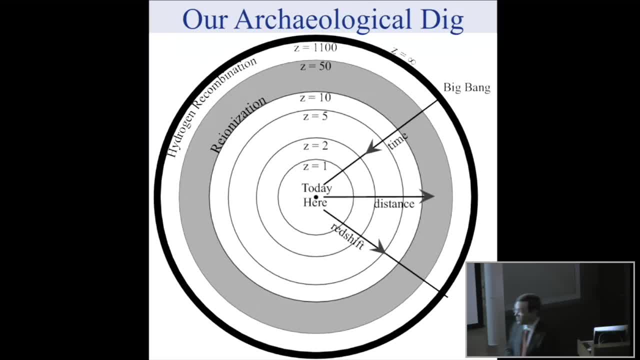 That's the maximum distance that we can observe things to, But, as it turns out, the universe was opaque early on and that's illustrated by this dark sliver, And we cannot use radiation to look through the universe at this very early time, when it was opaque. 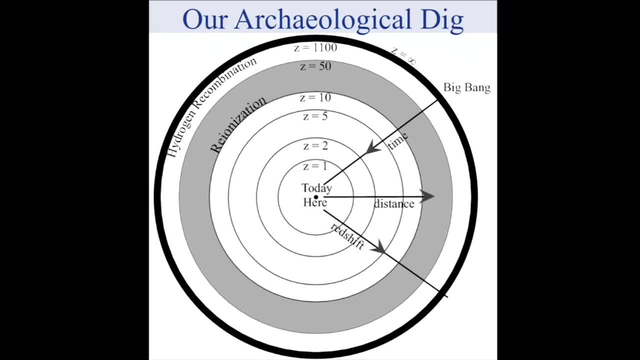 But what we can see is the photosphere from that surface, similar to the photosphere of the sun. The outer edge of the sun that we are observing has a temperature of close to 6,000 degrees Kelvin- The photosphere of the universe. 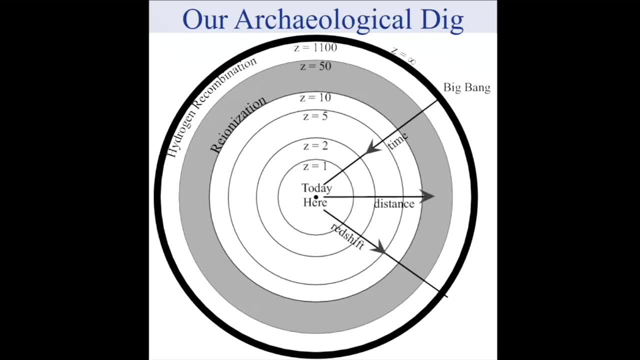 has a temperature which is quite similar to that of the order of 3,000 degrees and 3,300 degrees Kelvin, And we can see this photosphere, We can see the radiation coming from it, and that's called the cosmic microwave background. 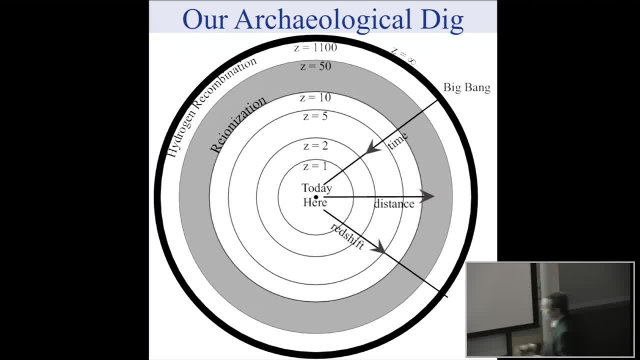 That's the time in the history of the universe when the universe became transparent. So, starting from this photosphere and closer to us, we can actually observe the universe. Now you may ask how far have we observed it so far And the surveys that we have? 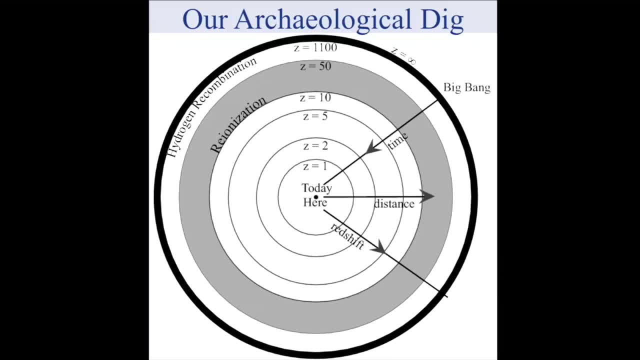 of matter go out to scales that are relatively close to us. A few years ago, we only surveyed about a tenth of a percent of the volume of the universe. By now we are serving maybe a few percent of the volume of the universe. 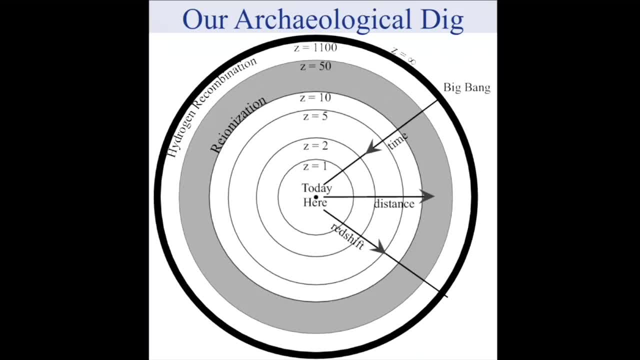 You realize that the volume goes as distance cubed. So as you go to earlier times you're actually probing most of the volume of the universe And for professional astronomers that corresponds most of the observable volume of the universe in moving coordinates. corresponds. 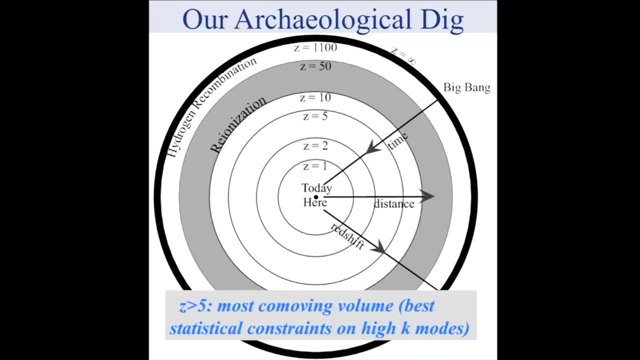 to redshifts above five. And the reason that's attractive to observe those early times is because we get the biggest sample of independent regions that can tell us about the initial conditions of the universe. So if you want to know to a very high precision, 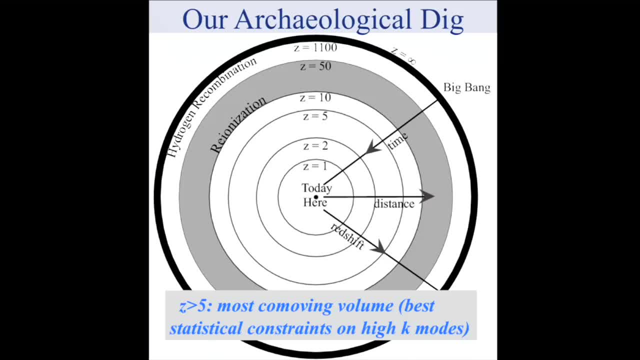 what the initial conditions of the universe were. we really want to go to early times, when these conditions were imprinted in the universe, but also because the volume that we can see is much larger at earlier times than it is closer to us at late times. 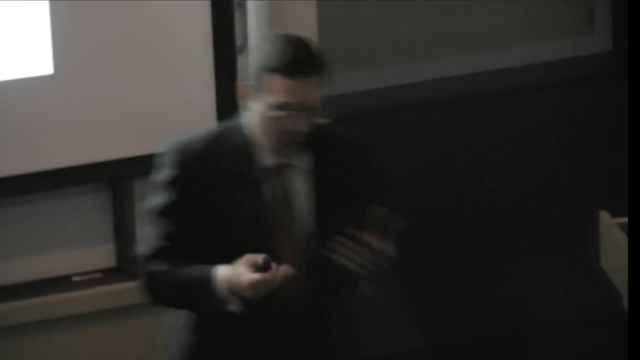 And that's an important reason for why we want to go to high redshifts or early cosmic times. So far, if we look at the photo album of the universe that we have, we have this first image, that of the cosmic microwave background. 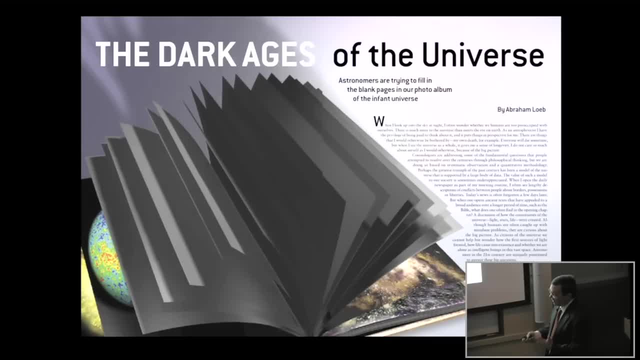 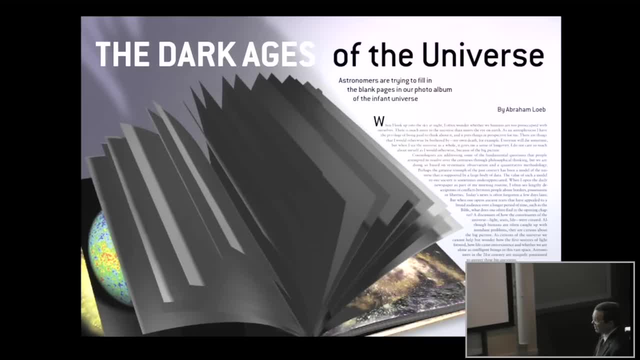 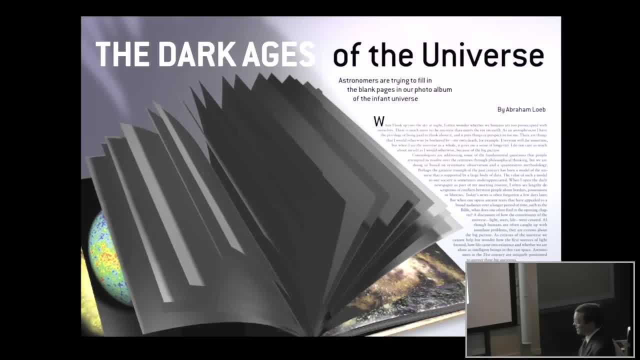 became transparent And a billion years is when galaxies as big as the Milky Way were formed, And we would like to fill in these missing pages in our photo album. And, as we all know, an adult is not just a scaled-up version of an infant. 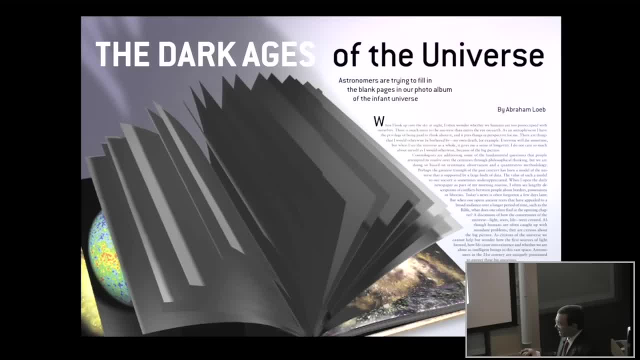 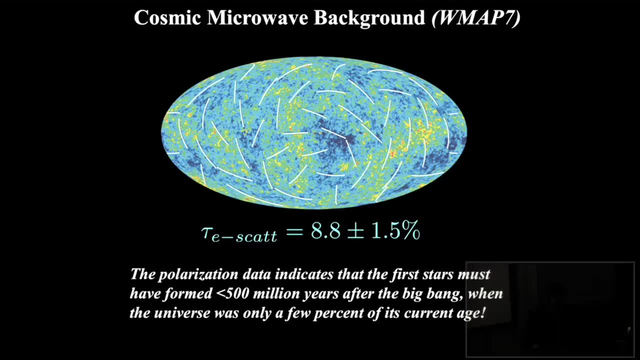 And therefore it's not a simple extrapolation. correlation between the initial conditions and the final state And the cosmic microwave background is really the Rosetta Stone of cosmology. It allowed us to figure out the initial conditions that existed in the universe at the redshift. 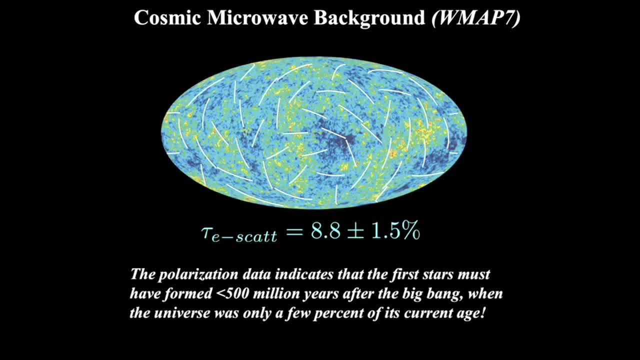 of 1100, 400,000 years after the Big Bang, when the universe became transparent, And by analyzing the polarization of the microwave background on large scales, we're able to conclude that the first stars in the universe must have formed less than 500 million years. 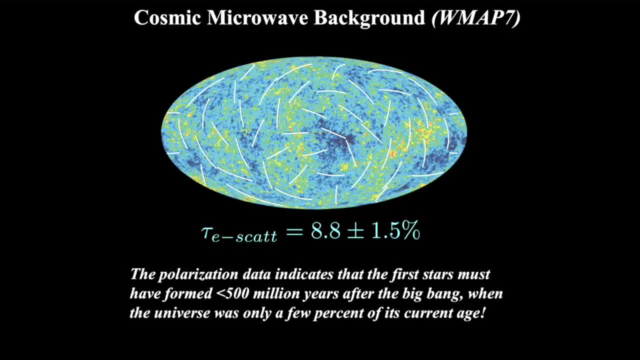 after the Big Bang, because they broke the hydrogen atoms into their constituent electrons and protons, and the electrons scattered the microwave background once again. About 10% of the microwave background photons that we see were scattered by electrons that were released due to the ultraviolet radiation from the first stars. 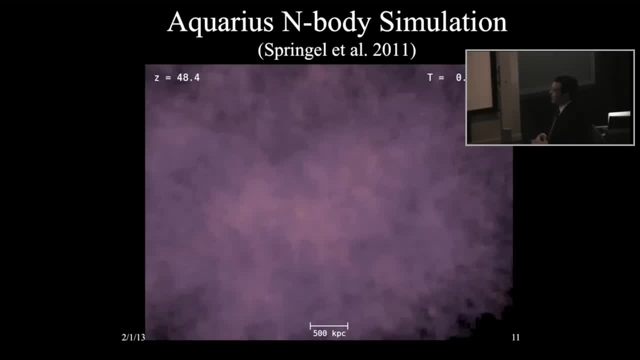 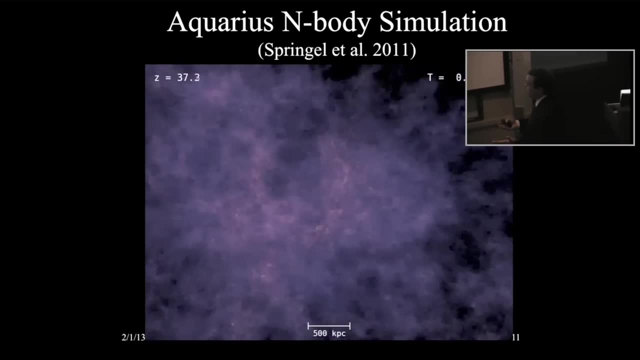 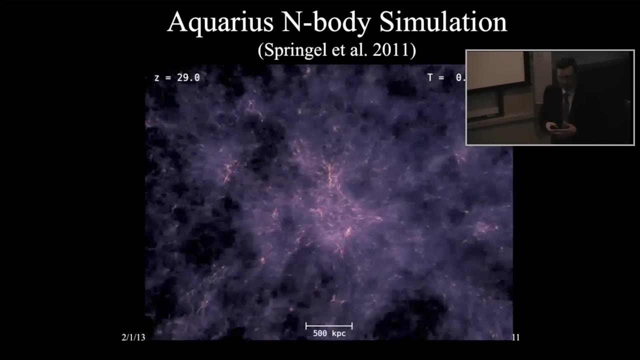 So that we can conclude- And we can in principle start with the initial conditions- that we read off the cosmic microwave background and put it into a computer simulation that follows the dynamics of matter in the universe. Most of the matter in the universe is dark matter. 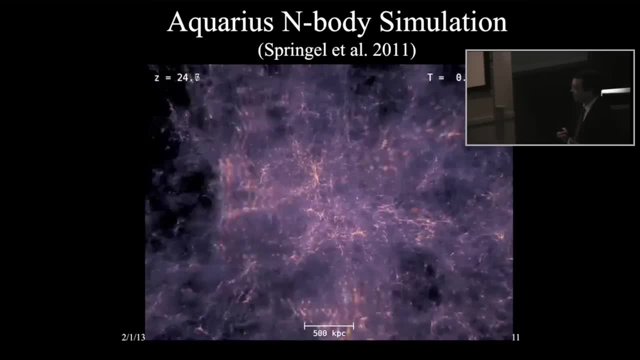 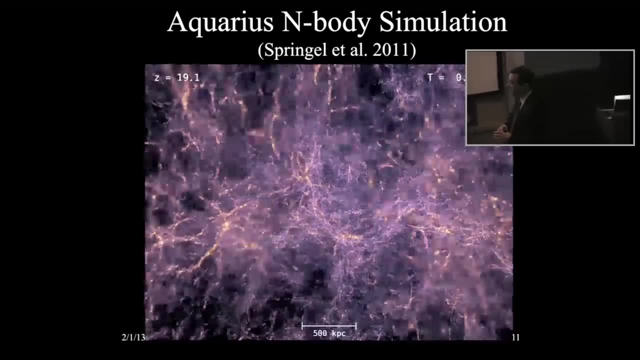 We don't know what it is, and it's quite surprising that we're getting paid as cosmologists even though we don't know what most of the matter is. It's not a matter that our bodies are made of. This matter does not interact with light. 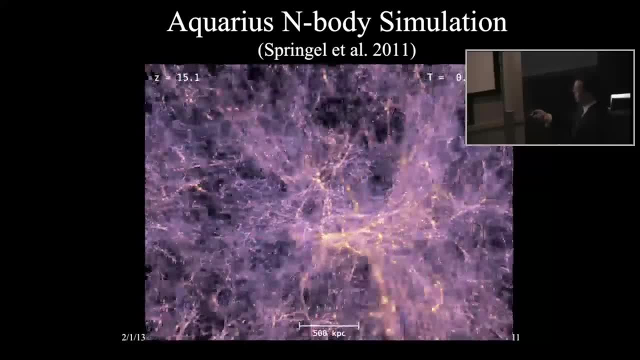 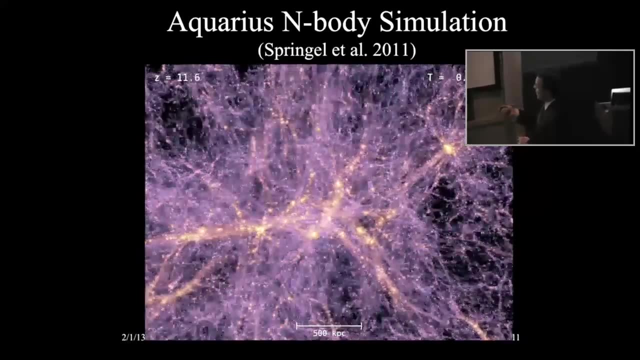 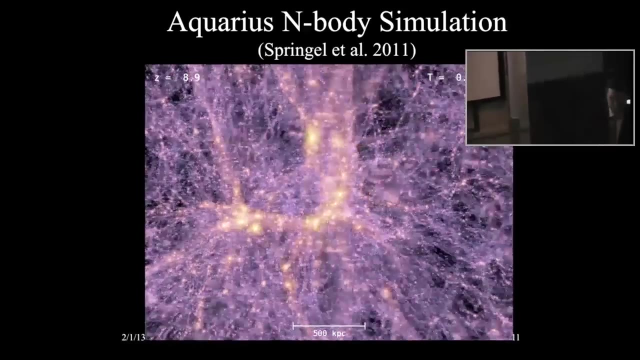 So we cannot observe it directly. But what we see is when we put the initial conditions into simulations that employ the laws of motion, we end up making these giant structures that in fact Margaret Geller, here in the audience, was the first to discover observationally. and we see those filaments. 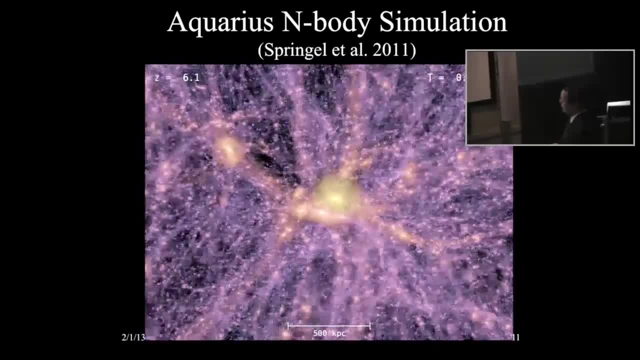 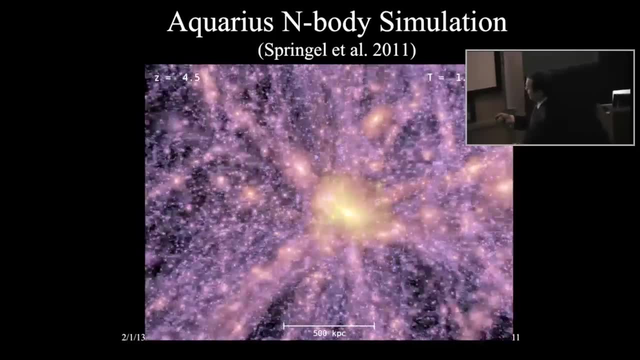 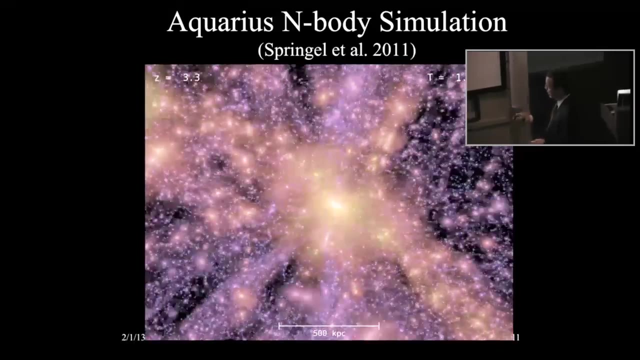 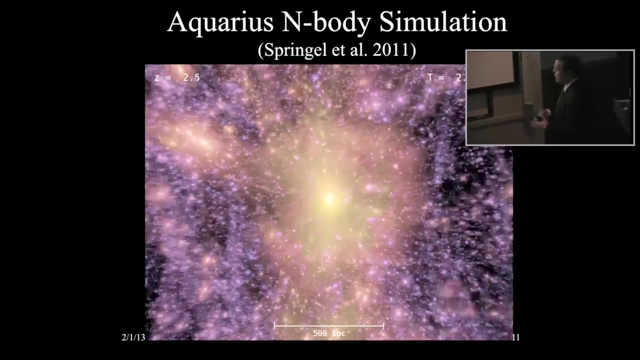 and sheets that describe the cosmic web And you see an enormous number of small clouds of dark matter called hellos. The bigger ones are actually representing big galaxies, the smaller ones are small galaxies And there are some dark matter clumps that do not have stars in them, because when we 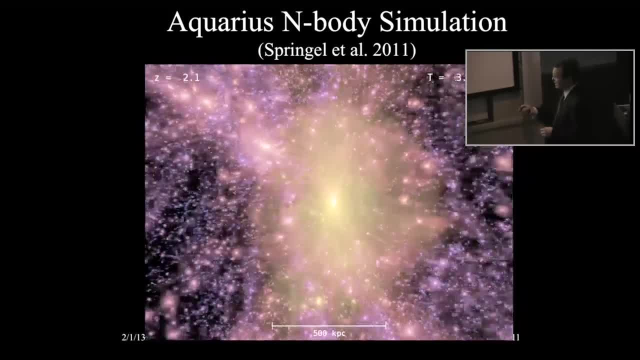 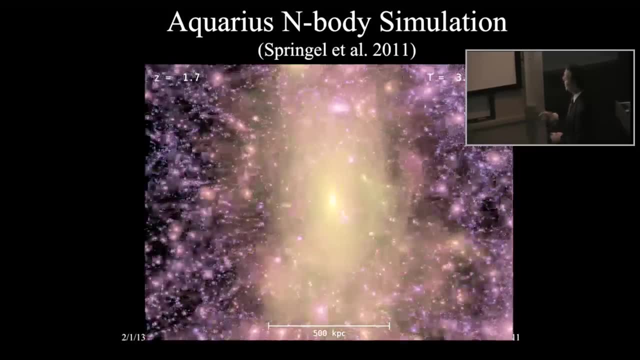 count the number of galaxies, we see far fewer galaxies than the number of dark matter clumps in these simulations And this is just the behavior of the dark matter. And you can see here the clock ticking in terms of the age since the Big Bang: the age 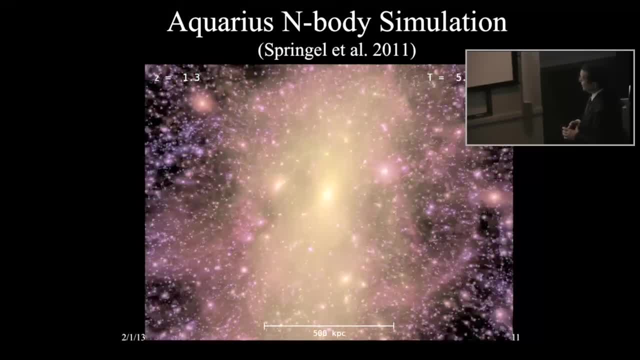 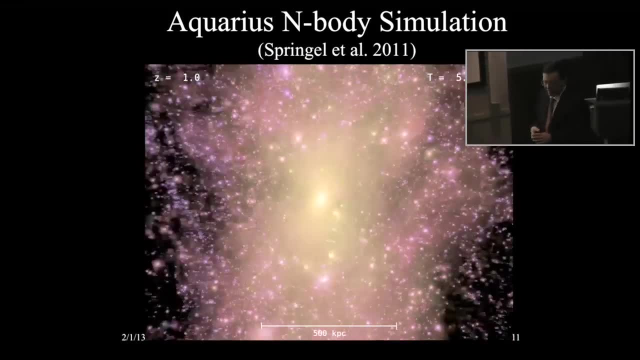 of the universe. The present age is 13.7 billion years, Structure starts to form very early, and the first galaxies formed around 100 million years after the Big Bang. Of course, the interesting question is once you put ordinary matter into these simulations. 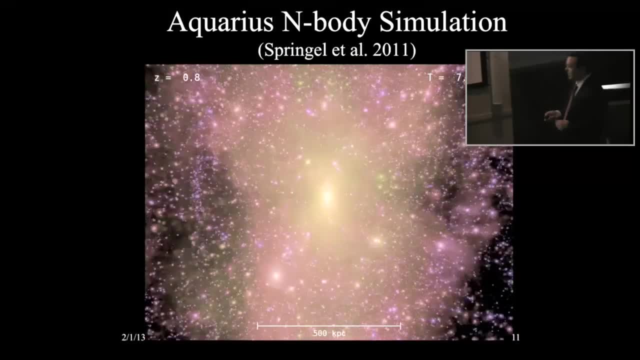 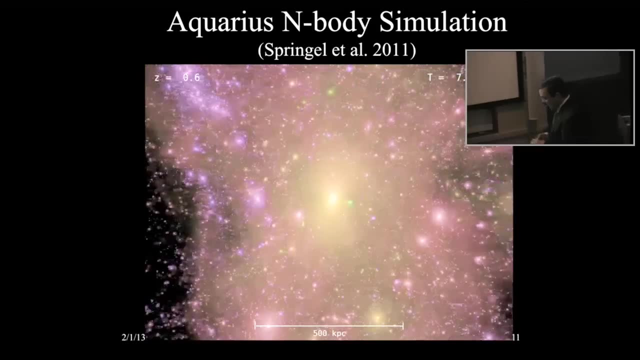 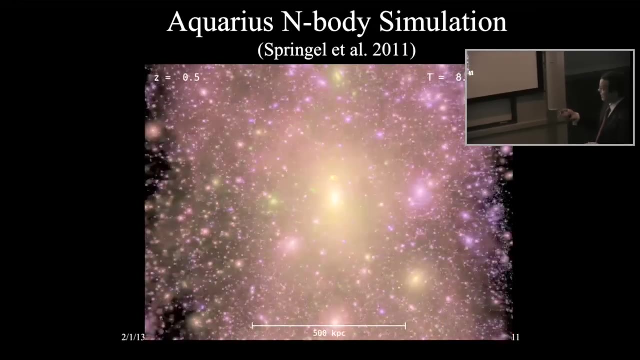 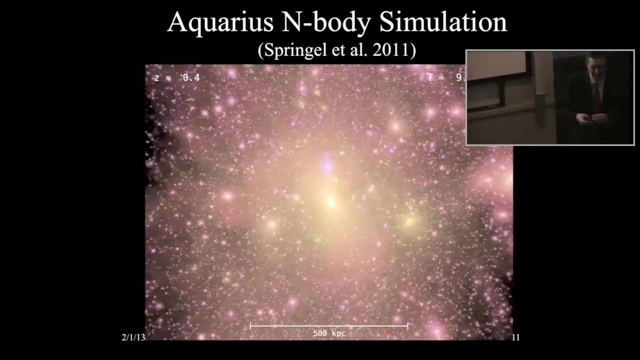 do we get galaxies that look the same as the galaxies before? Do we see any changes in the dark matter that we now see? And the problem, the real challenge of cosmology is that we can calculate very accurately what we cannot see. We can calculate very accurately what the dark matter is doing, because it's a very 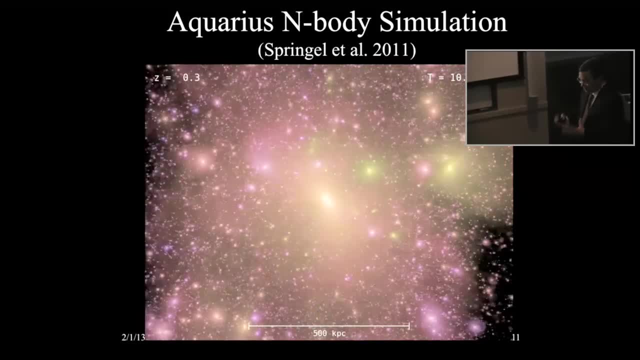 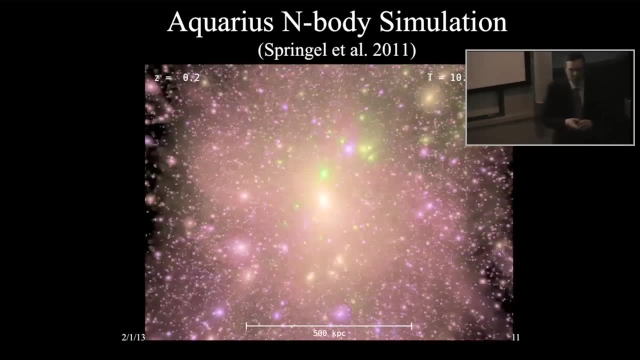 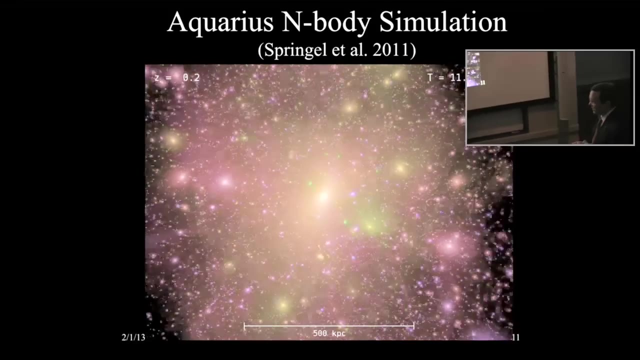 simple type of matter in our model right now. So we calculate extremely precisely what we cannot see in what we can see, the ordinary matter. we are unable to calculate it very precisely because of the complexity And that's an unfortunate situation. On the other hand, it allows theorists to shove all the problems with the dark matter. 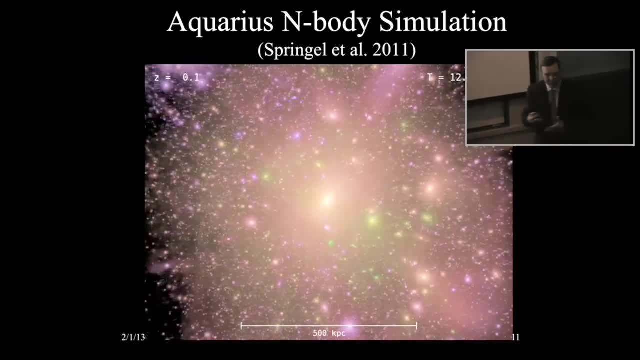 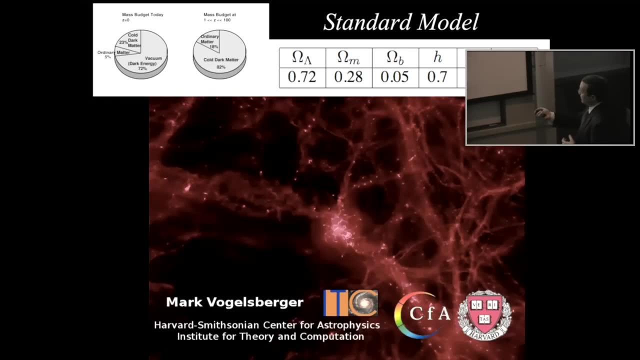 under the rug of the ordinary matter, They might say. well, the reason we don't get agreement is because the ordinary matter is not fully understood. And here is a simulation that does include ordinary matter and we are looking at a snapshot from different directions. 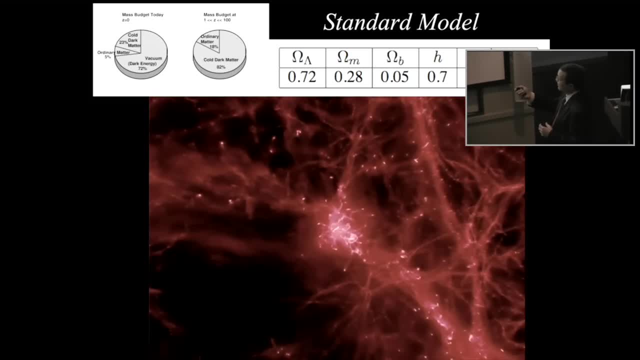 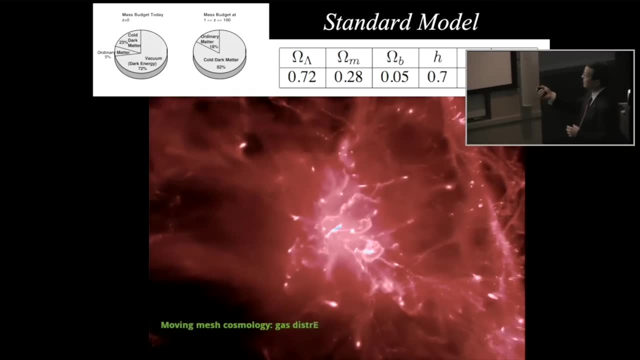 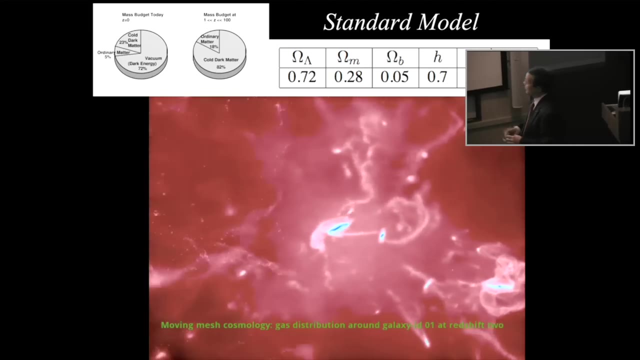 The standard cosmological model includes 28% of the mass density of the universe in the form of cold dark matter, only 5% in the form of ordinary matter, and 72% of it right now is in the form of the vacuum, the cosmological constant, or dark energy as it is called. 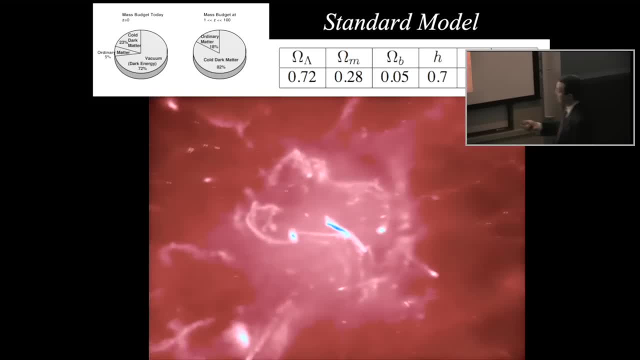 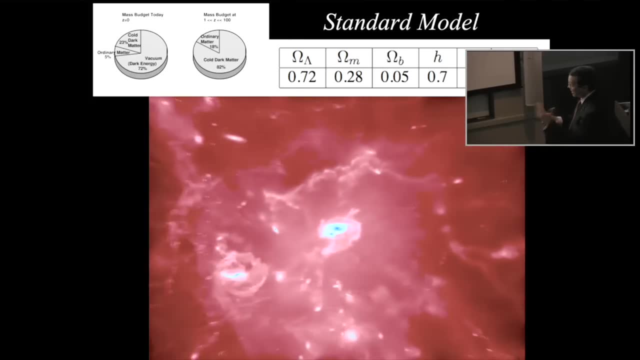 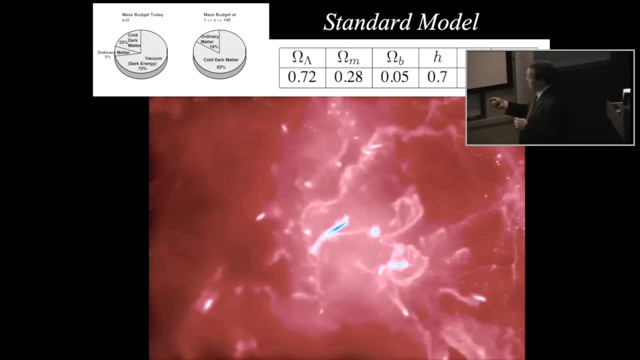 So that's the situation today And you see here the results of the simulation. This is a simulation that includes ordinary matter which leads- this is a state-of-the-art simulation done here by Mark Vogelsberger and Lars Hernqvist and collaborators- where- 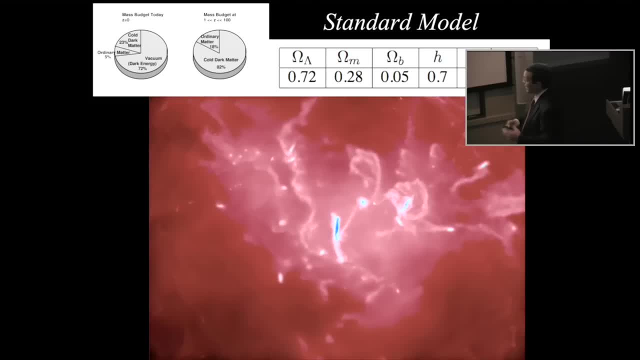 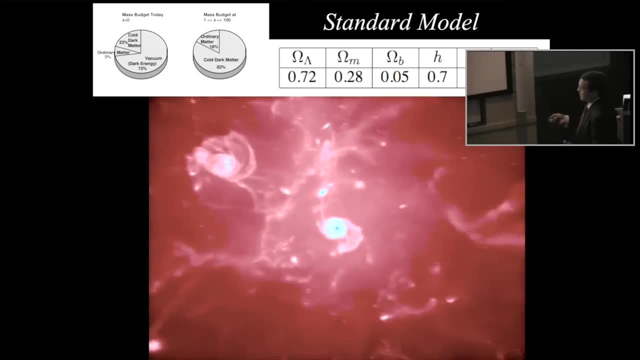 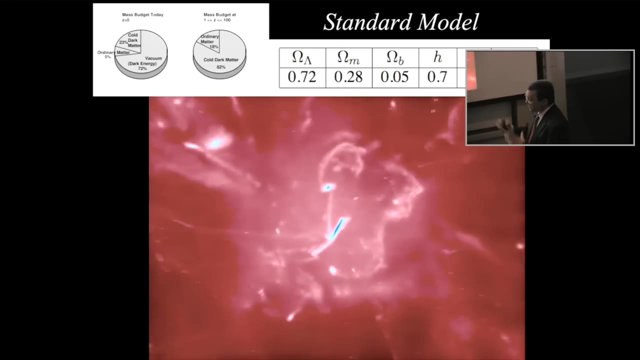 they did make a disk galaxy that looks just like the Milky Way. It has spiral arms and it has the right size and it looks similar to galaxies that we see around us. So the situation today is that the vacuum dominates, And that's why the universe is entering cosmic acceleration. The expansion of the universe is speeding up. it's not slowing down due to the vacuum, But as you go back in time, once you go beyond the redshift of one, when the universe was less than half of its present age, matter dominates. 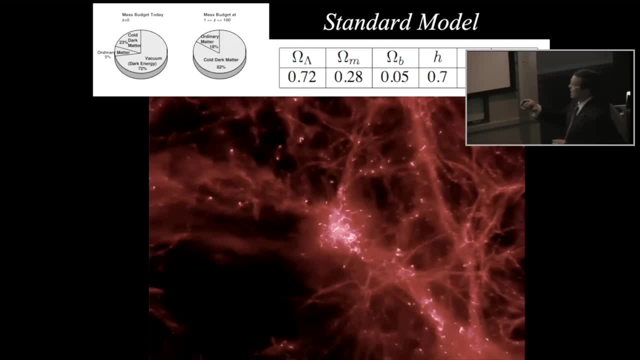 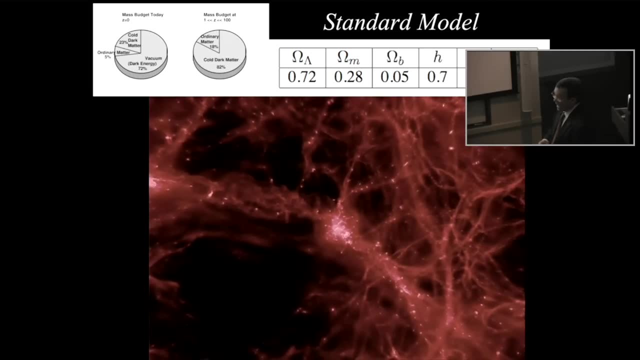 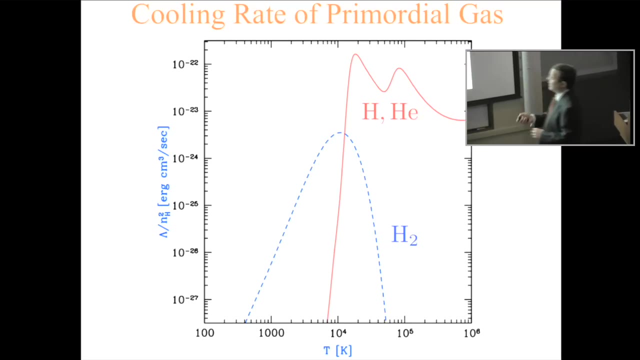 The vacuum is irrelevant at those early times and the cold, dark matter makes up 82% of the matter content, With ordinary matter making 18%, And that's what's relevant for the formation of the first galaxies. This plot shows the cooling rate of primordial gas, the gas that was left over from the Big 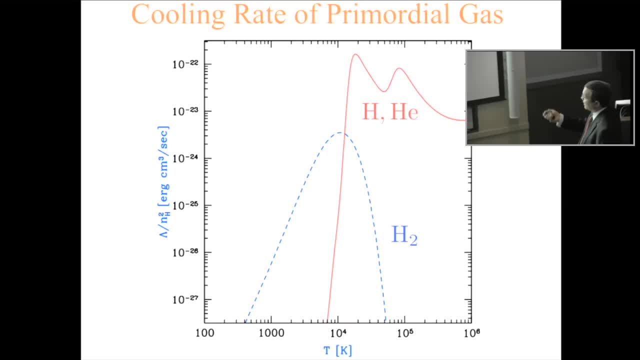 Bang, including mostly hydrogen and helium, as a function of its temperature, And the one prominent feature in this plot is that the cooling rate drops dramatically at temperatures below 10,000 degrees Kelvin, Meaning that Gas is unable to cool once it reaches this temperature floor of 10,000 degrees, unless 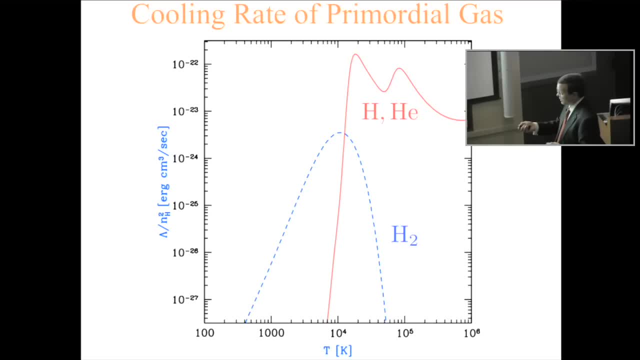 there is molecular hydrogen that allows it to cool, to lower temperatures, And that's very important because if you're making helos in which the characteristic temperature is below 10,000 degrees, you have to rely on molecular hydrogen allowing the gas to. 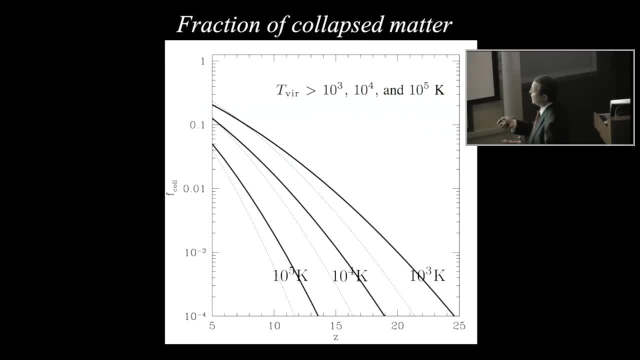 fragment into stars, And you may ask which fraction of the matter in the universe collapsed into helos Above 10,000 degrees Kelvin, And the answer is at redshift 10, when the universe was 500 million years old, only a. 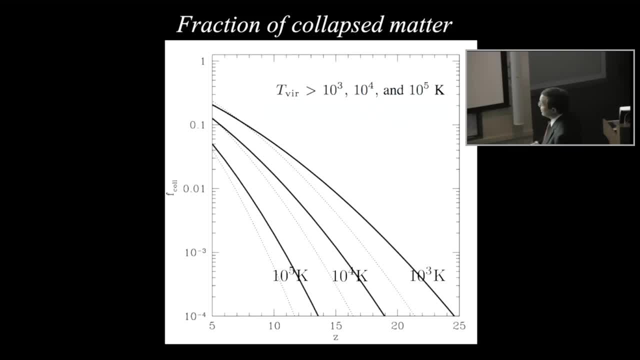 percent or so of the matter was incorporated into objects that had high enough temperature to fragment. For the gas to fragment into stars through atomic cooling of hydrogen or helium. That's a small fraction, only 1%- But keep in mind that to ionize hydrogen you just need 13.6 electronvolts per hydrogen. 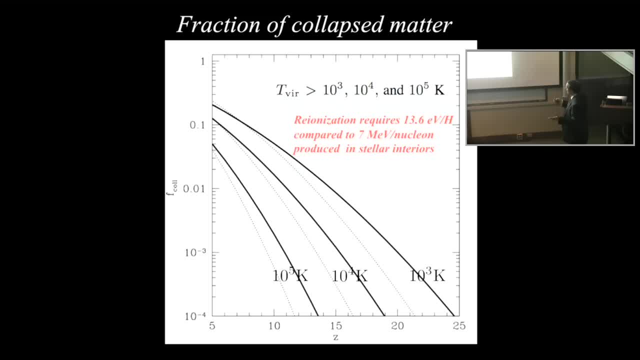 atom and that's compared to a number that is 5 to 6 orders of magnitude, almost a million times bigger that you get out of burning hydrogen in stellar interiors. So you basically just need to incorporate 10 to the minus 5, or a millionth, a few millionths. 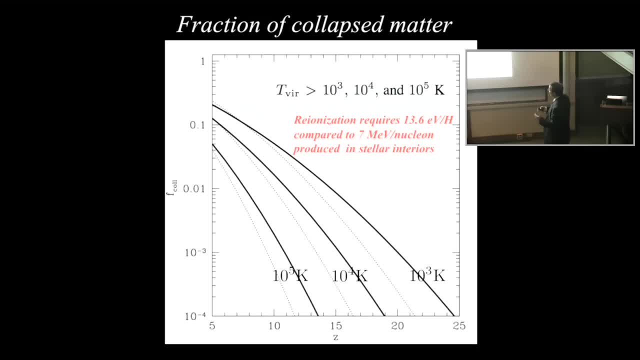 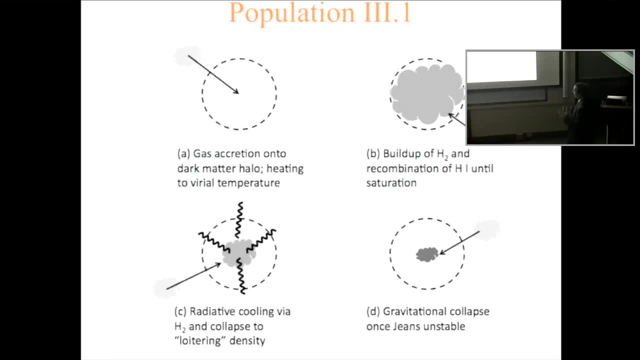 of the gas in the universe into stars And burn the hydrogen in order to ionize, to break the rest of the hydrogen in the universe. So how did the first stars form? The current theoretical model is illustrated here, starting from the cosmological initial. 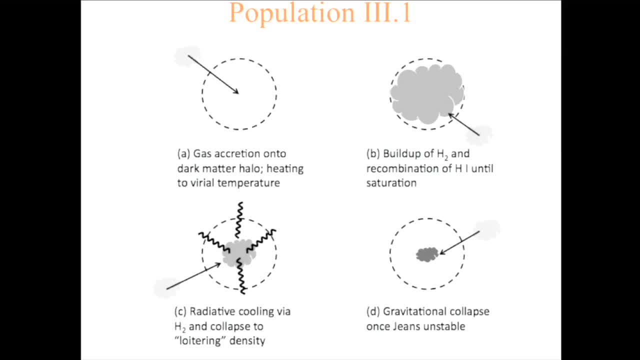 conditions: gas accumulated into clouds in which molecular hydrogen formed- and one can follow the chemistry of molecular hydrogen formation- and molecular hydrogen cooled to allow the gas to fragment, And that's how the gas went into the first, very first generation of stars. 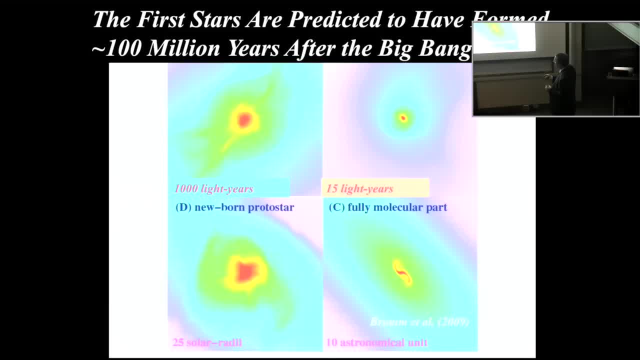 And numerical simulations can follow the evolution of these early gas clouds all the way down to the scale of a star, And what one finds is that the typical infall rate of mass onto such early stars is higher than it is today in our galaxy, for example, simply because the temperature, the characteristic 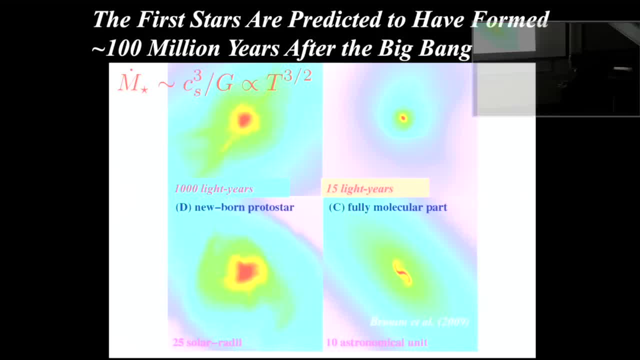 temperature of the gas was higher at earlier times. The cosmic microwave background was hotter And from dimensional analysis you can calculate the mass infall rate of gas onto these early stars and you find that, for the characteristic temperature that molecular hydrogen can call the gas to, you end up with masses that are about 10 times the mass of the Sun. 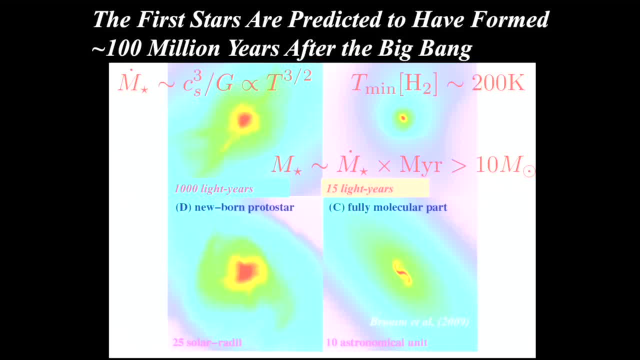 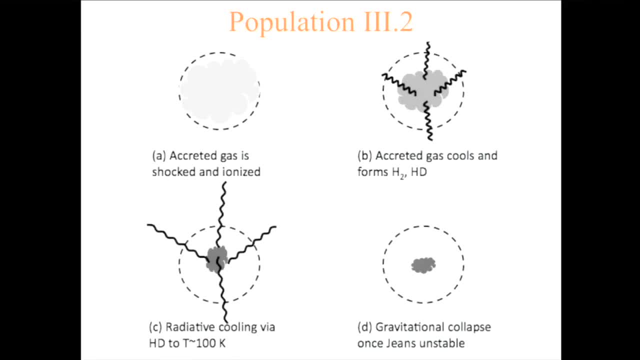 So these early stars were probably much more massive than the Sun, And then these first stars produced radiation that affected the gas around the Agriculture them and affected the way that the gas can cool And, in particular, once the ultraviolet radiation from these very first stars impacted the surrounding gas, 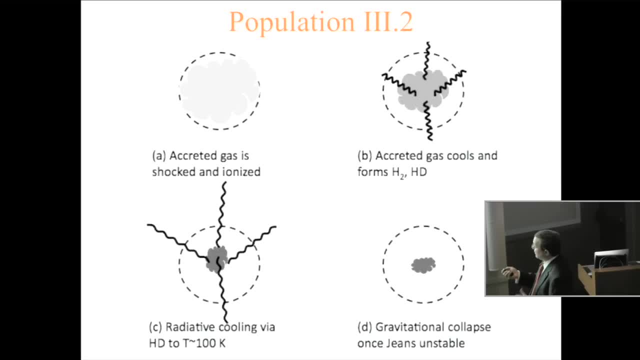 the gas was ionized, was broken into electrons, free electrons and protons, and other molecules could form, such as HD deuterium hydride, which is an asymmetric molecule. So the molecular hydrogen doesn't have a dipole moment, but the 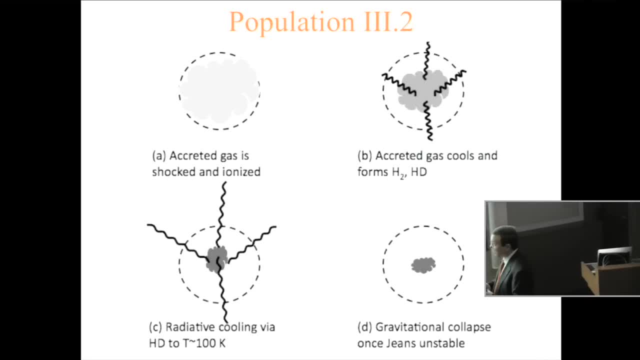 molecule like HD is a much more efficient coolant because it has a dipole moment and that allows the gas to cool much more effectively to temperatures down to a hundred degrees Kelvin where you can make low-mass stars. So this is called population 3.2.. The first population of stars was population 3.1.. 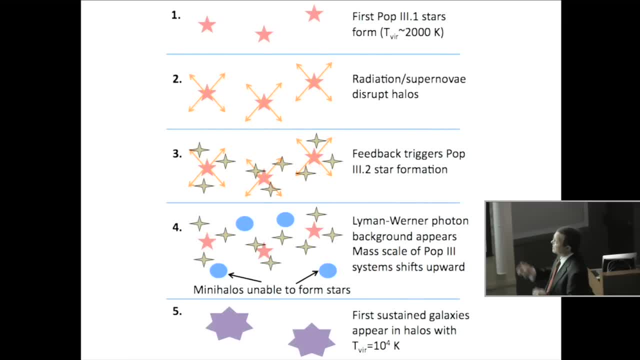 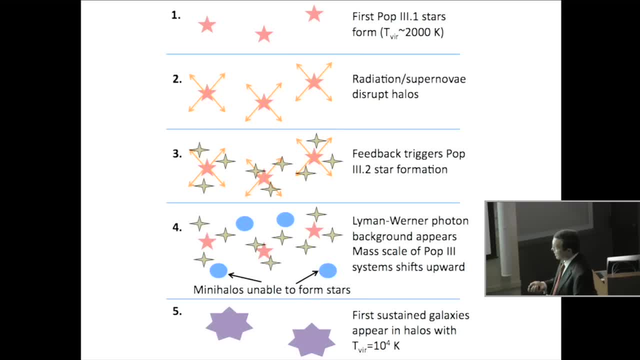 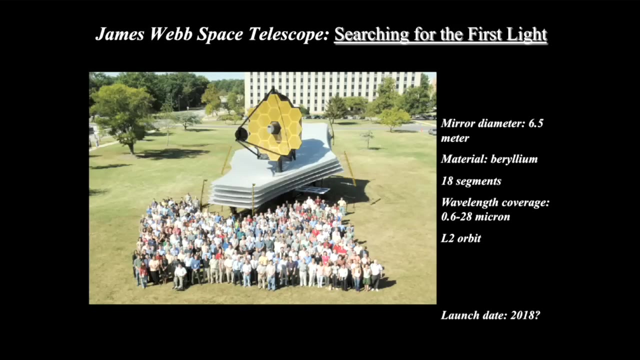 around them in a way that allowed lower-mass stars to form, And most of the stars that ionize the universe were actually made in hellos that had the temperature above 10,000 degrees Kelvin. Now the challenge is to observe the stars. 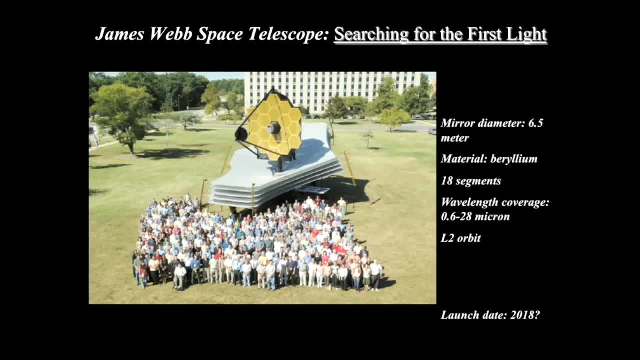 And the hope is, with a successor to the Hubble Space Telescope called the James Webb Space Telescope. It's expected to be launched in 2018, and I put a question mark because that depends on the approval from the Congress. It seems like this date is more realistic now than it was a few years ago. This telescope, 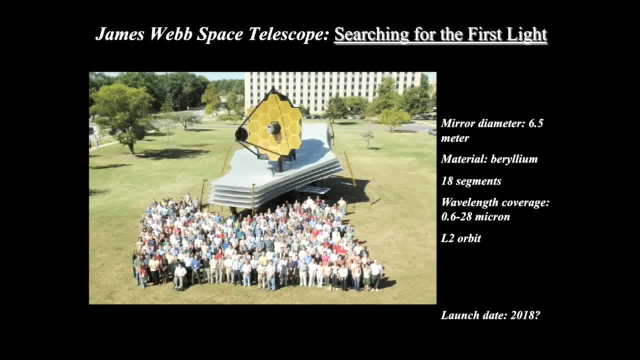 will have. this is a mock of the telescope. it will have a diameter for a mirror of six and a half meters and it will be in an L2 orbit. It will be sensitive to the infrared radiation coming from those early galaxies as it 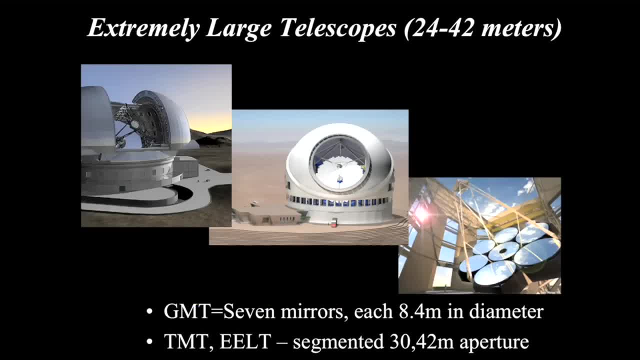 gets redshifted And, of course, there are plans to build big telescopes, the next generation of large telescopes on the ground. Harvard is a partner in the giant Magellan telescope that is illustrated here on the right, including several mirrors, each of which will be 8.4 meters in diameter, And you can see here the 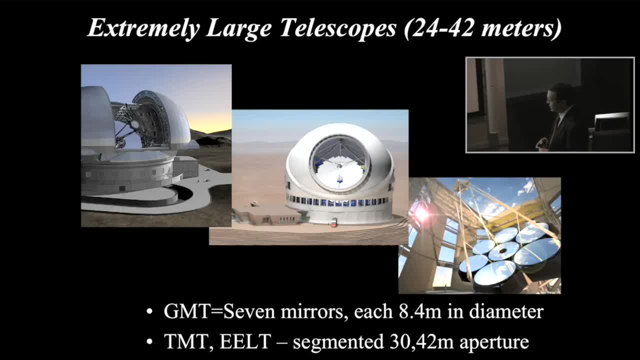 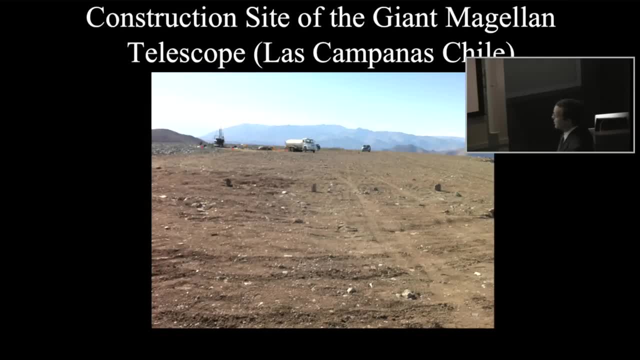 artist's conception. One of these mirrors was already made. the second one was also made. the third one is on its way, And this is a picture taken on Monday. I was at Las Campanas Observatory in Chile, and that's where the giant Magellan. 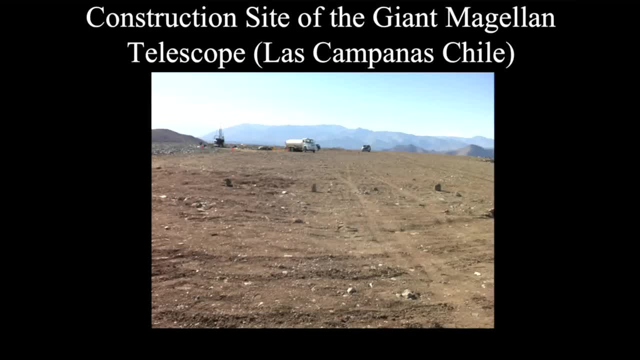 telescope is expected to be constructed And this is the top of the mountain where it will be situated. It was flattened by an artificial explosion last year and it looks very flat right now- the size of two football fields. It looks very impressive And I'm 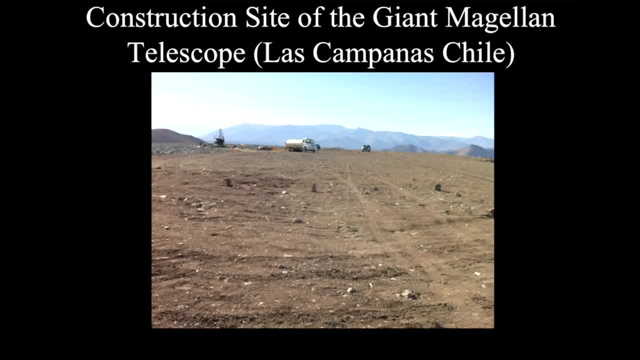 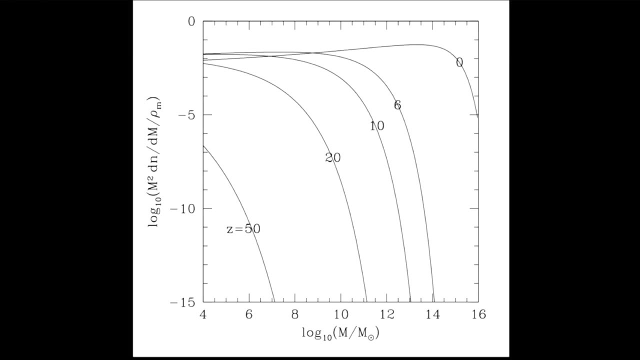 just starting now with the plans of, how you know, putting things in place and, subject to the approval by the board of the giant Magellan telescope, to move ahead with the construction. Now, as I mentioned, we can calculate the properties of the dark matter quite accurately. 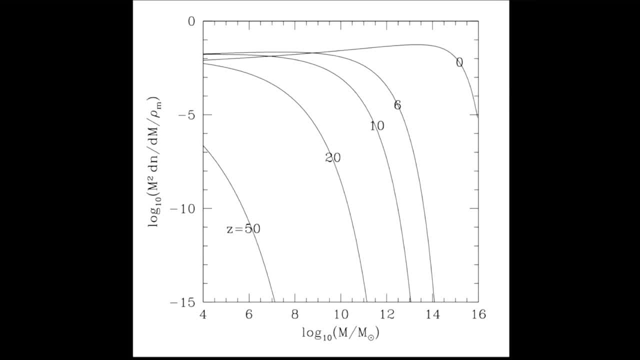 and one property that we are particularly interested in is the number of dark matter halos as a function of their mass, And what I'm plotting here is the amount of mass in dark matter halos parallel to a rhythmic mass interval. So this beam here, for example, corresponds to 10, to the power 10 solar masses. The Milky Way galaxy is 10 to the 12 solar masses and we are looking at different redshifts here Early times, at early times. the very few galaxies, in fact there are no galaxies with a mass like the Milky Way at 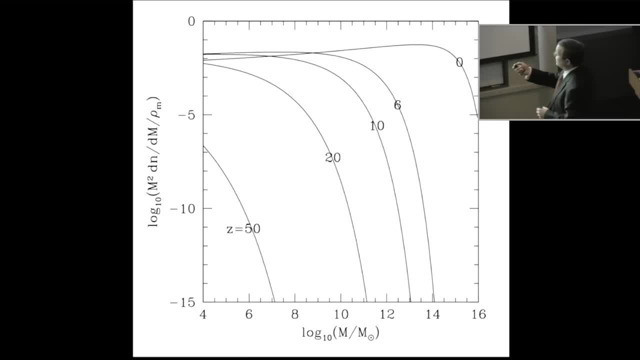 the redshift of 50. But as you go down to redshift 10, they start to appear And what you see from the top here is that there is roughly equal amount of mass parallel to the rhythmic halo mass beam, And the present day is marked with the formation. 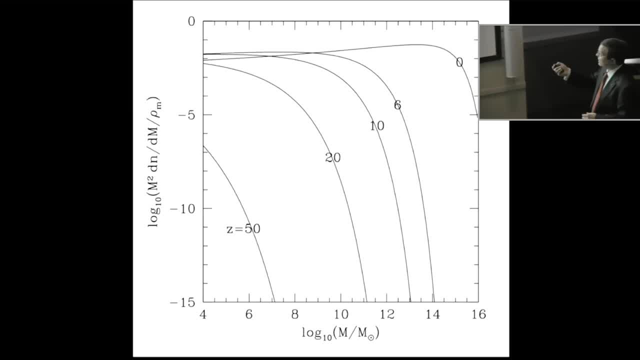 of groups of galaxies or clusters of galaxies. If you go to earlier times, you then the characteristic mass halo. mass in the universe goes down And galaxies like the Milky Way were made around the redshift of a few. When we look at 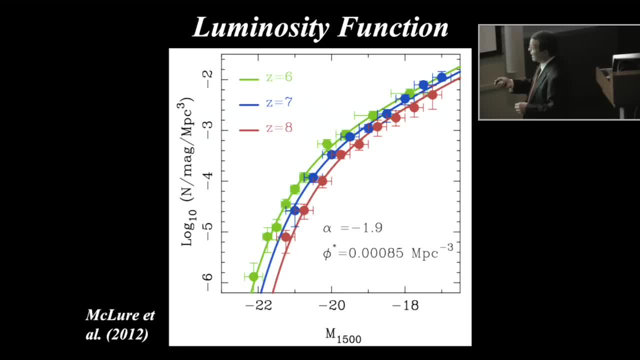 galaxies. these are the latest results of the number counts of galaxies. We also find an interesting analogy to the mass function of halos. We find that there is equal amount of light parallel to the rhythmic light interval in the luminosity function of halos. 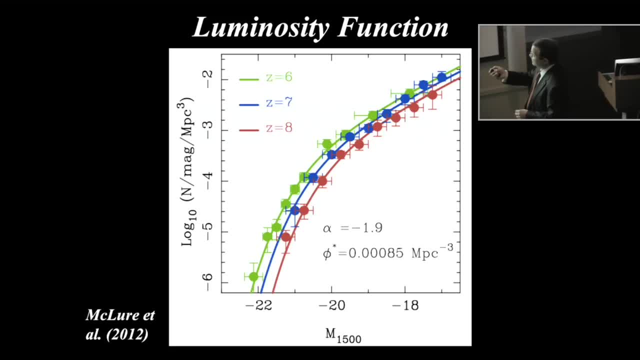 Galaxies, and what I have here is the luminosity function of redshift 6,, 7, and 8, as measured from the Hubble Space Telescope observations. So, interestingly enough, there is equal amount of light parallel to the rhythmic light interval. that matches what you expect for the halo. 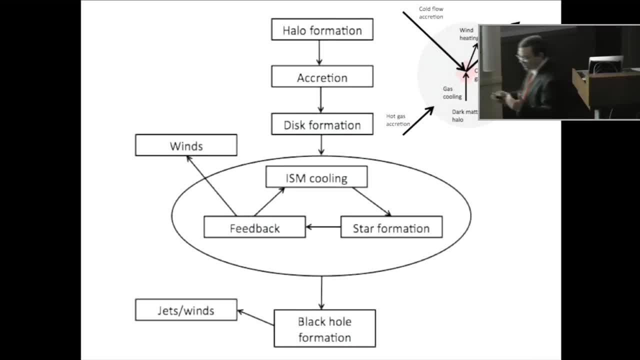 mass function. So the mass to light ratio appears to be constant in those early galaxies. And when you make a galaxy, there are several ingredients to the recipe that you need to use, And that's why galaxy formation and evolution is a complex subject. First of all, the easiest part to 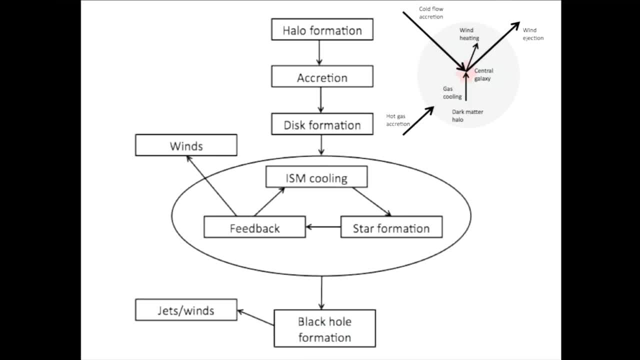 understand is how the dark matter halo forms and you can even understand it analytically, and that is described in the book. But once the dark matter makes the halo, the dark matter halo gas assembles into that halo and the gas is able to cool and settle to the middle. 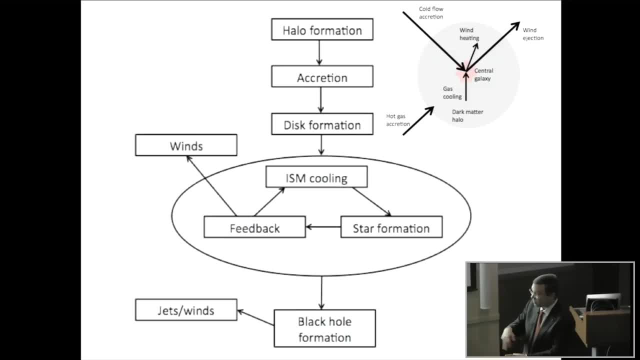 of the halo, where it's held against gravity by its rotation, by the centrifugal force, And that's where the gas forms a disk. And inside the disk there is gas that can cool, make stars, and the feedback from those stars can send out winds from the galaxy. so the 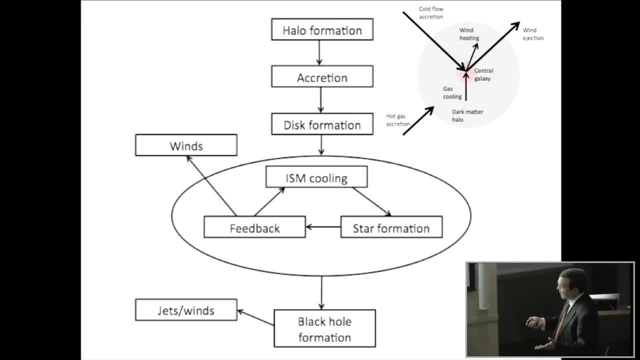 gas is being recycled And then in the center of the galaxy a black hole may form and the black hole again can make jets and winds and affect the galaxy, And that's where the subsequent evolution of the galaxy is, And so the feedback from the star formation and 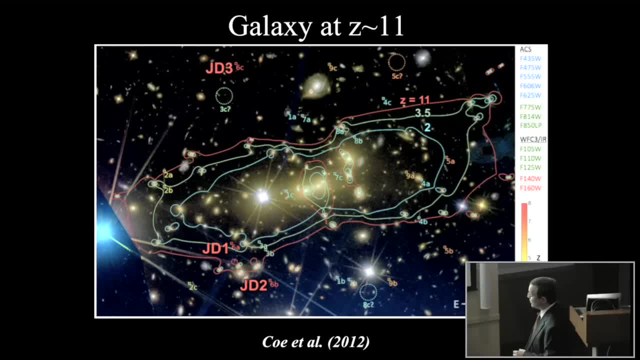 the black hole formation makes galaxy formation a complex subject. It's self-regulated. The highest-gratitude galaxy that was reported back in November 2012 used an artificial well. we used the Hubble Space Telescope to look at a cluster of galaxies which acted. 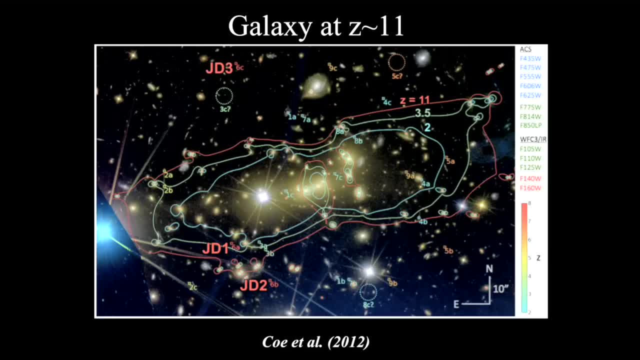 as a gravitational lens. So we're using nature to help us get an image of a very faint galaxy in the background, And so the cluster of galaxies focuses the light from a background faint galaxy and serves as a gravitational lens Due to its gravity. we end up getting three. 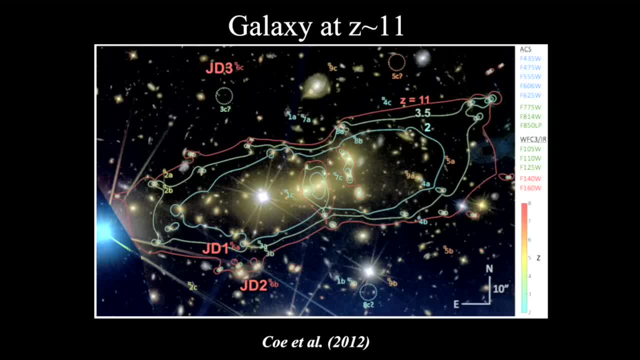 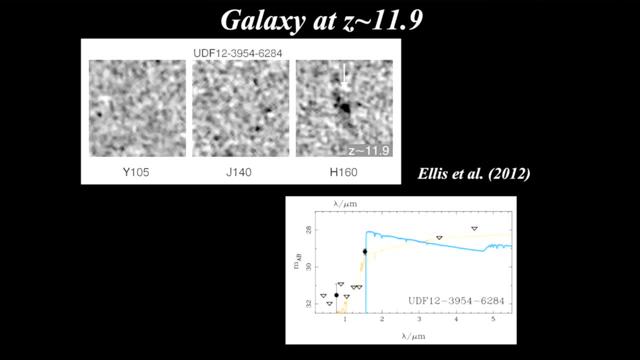 images of this background galaxy, which is inferred to be a correction of 11.. But then, a month later, there was a report on a galaxy at a redshift of 11.9, potentially again from data that was collected by the Hubble Space Telescope in September 2012.. 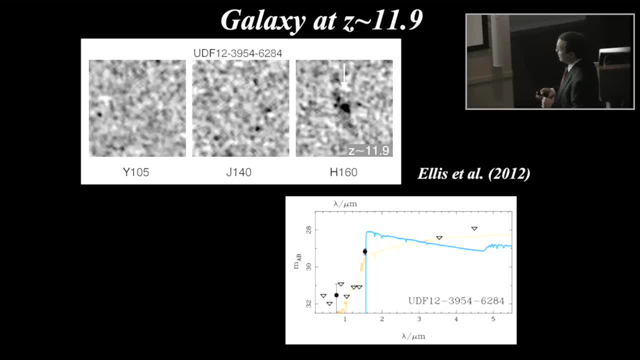 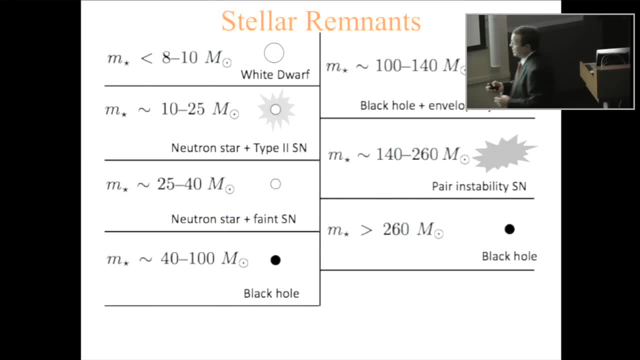 So currently this is the record holder, and there is some debate about the reality of this redshift determination. When stars form, they of course burn and eventually they actually consume their nuclear fuel. And of course, an interesting question is: what's? 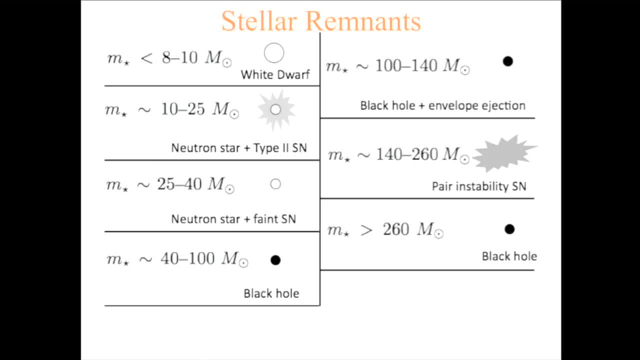 left behind. If the stars are very massive, as the first stars were, they can leave behind either a neutron star or a black hole. or if they have a mass between 140 and 260 times the mass of the Sun, they produce a new type of supernovae called peristability supernovae. 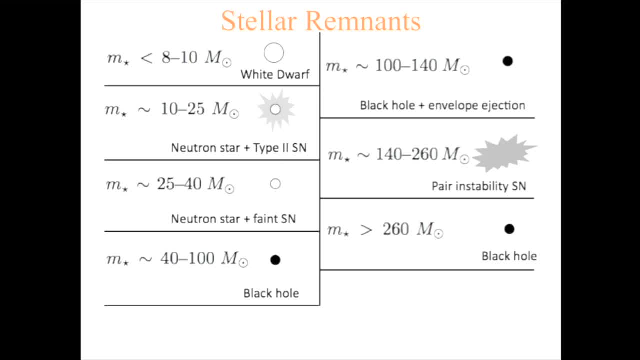 These supernovae were understood already back in the 60s by a group of Israelis, and they may wonder why they were worried about explosions back then. And for the very first stars, these supernovae were probably quite important because they enriched the gas with heavy elements that we are made of, like carbon or oxygen, and 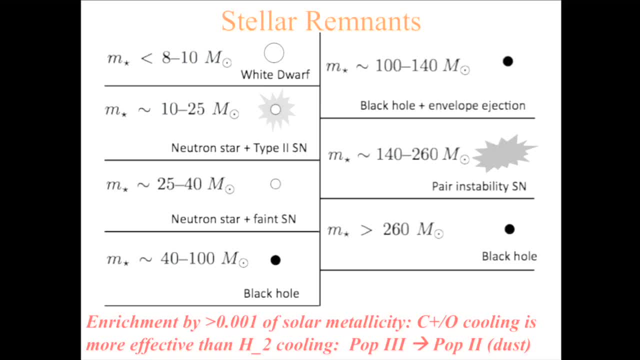 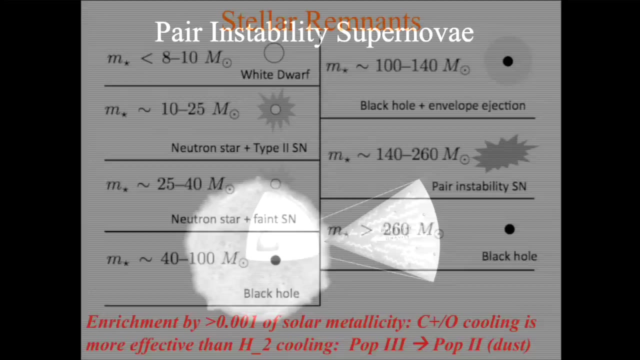 if you enrich the gas even by a tenth of a percent of the abundance of heavy elements in the Sun, then you find that 4.10% or oxygen cooling is more effective than molecular hydrogen. So it was very important for this enrichment to take place in order to allow the gas to 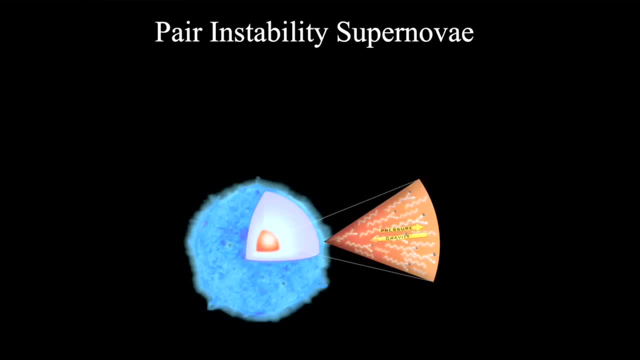 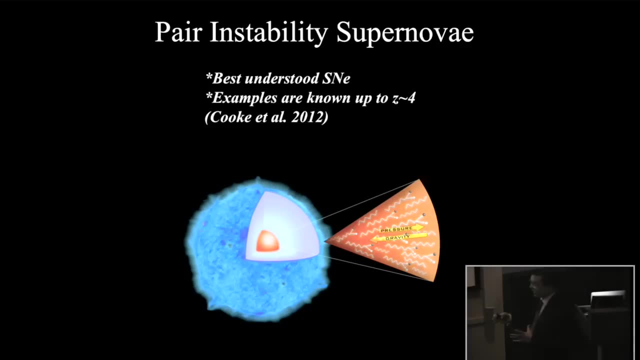 cool into low mass stars And peristability. supernovae have a very simple mechanism, The only type of supernovae that are fully understood. the explosion mechanism is fully understood and one is dealing with a massive star that consumes its nuclear fuel and then 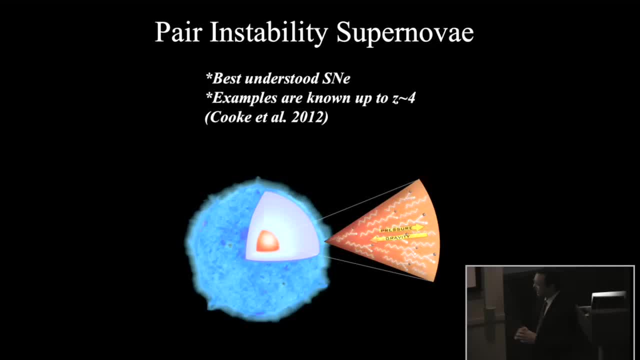 contracts and the temperature in its core rises to a level that allows electron-positron pairs to form. The temperature is so high that the star makes electron-positron pairs. the pressure drops and then further collapse and eventually explosion takes place. There is no remnant left behind in these explosions. 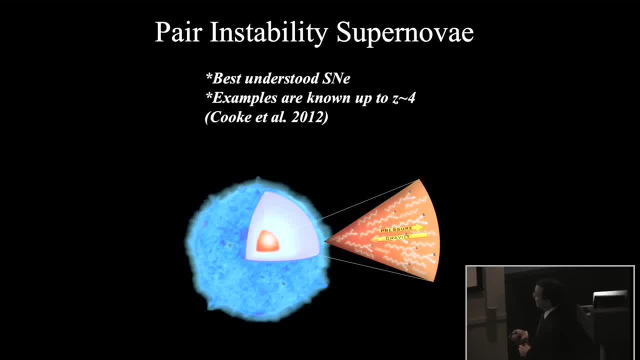 And there are examples that were just reported last year of candidates for peristability supernovae up to RETCHI-4.. The amount of energy that you get out in these supernovae is about 100 times the energy that you get in a normal supernova. 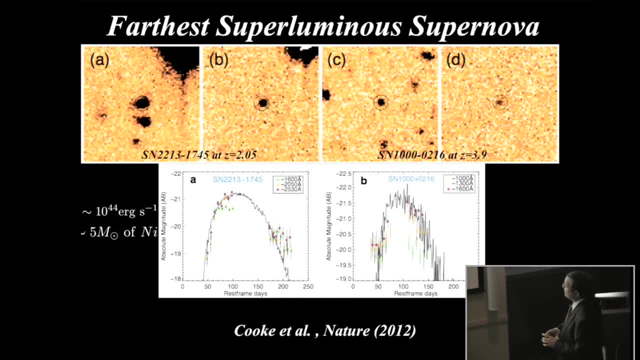 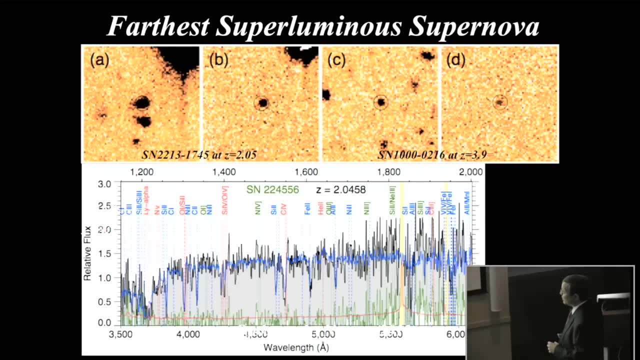 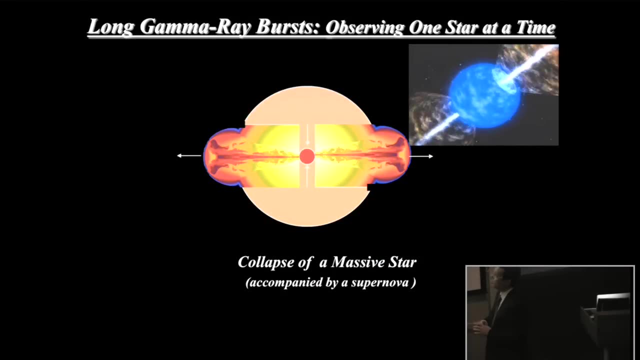 And these are the finding charts for the farthest supernova that was found at RETCHI-4 of 3.9.. It was reported in Nature last year. Another type of objects that result, or sources that result from, are stellar objects. 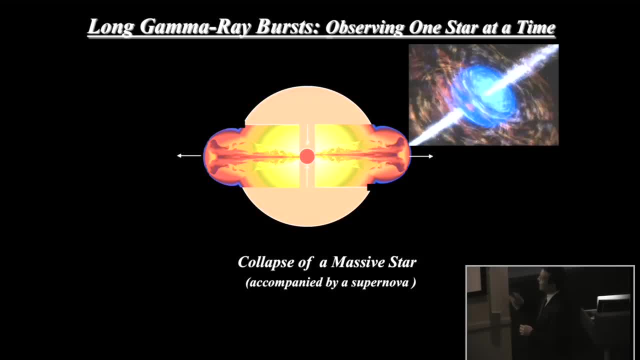 One of them is gamma-ray bursts, And here one is making for long duration gamma-ray bursts, one is making a black hole as a result of the collapse of a core, the core of the star, And then during that process, jets are being produced, just like the jets we see in extra-galactic. 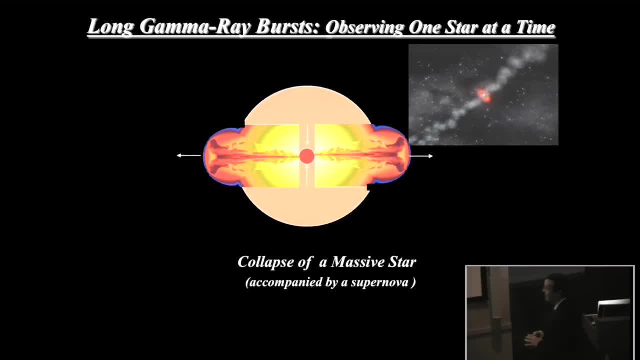 or large, massive black holes at the centers of galaxies outside of the Milky Way, And these jets are drilling at the center of the Milky Way, And these jets are drilling at the center of the Milky Way And when we see these jets we have a hole in the envelope of the progenitor star and 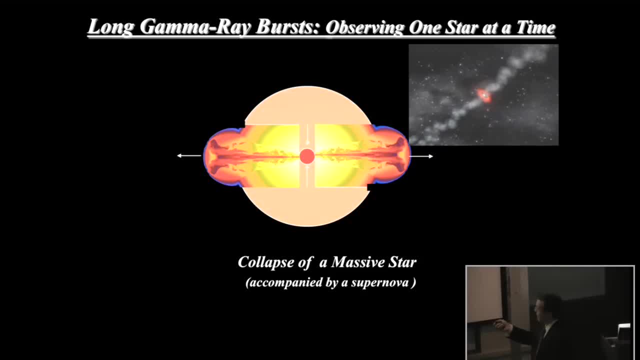 eventually exiting from that envelope to be seen by an observer that is aligned with the axis of the jet. And when an observer looks at such a jet, the time is being contracted. The emission is seen as a flash in gamma-rays And these are called gamma-ray bursts. 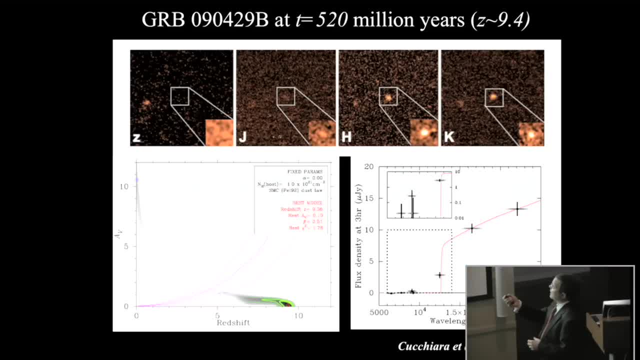 And they, in principle, can be seen all the way to the edge of the universe universe. the highest redshift gamma-ray burst that was detected is from 520 million years after the Big Bang, almost at a redshift of 10.. 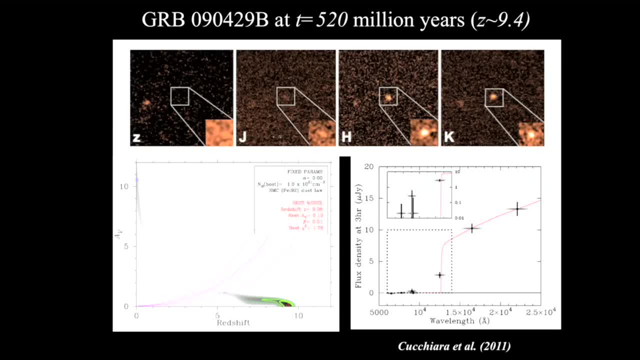 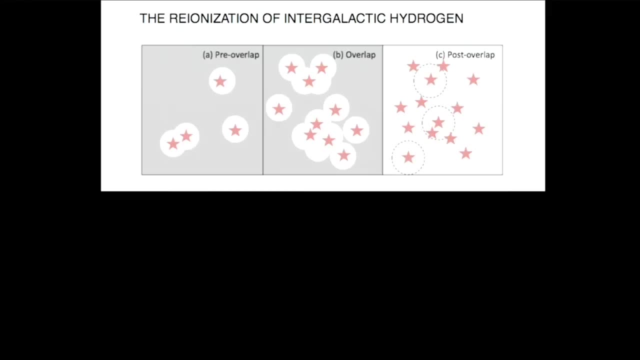 And for over a decade I have been advocating the use of gamma-ray bursts for exploring the first stars, because you are seeing one star at a time. How can we observe the gas in between the galaxies? Well, the reason we are interested in doing that is because the ultraviolet radiation 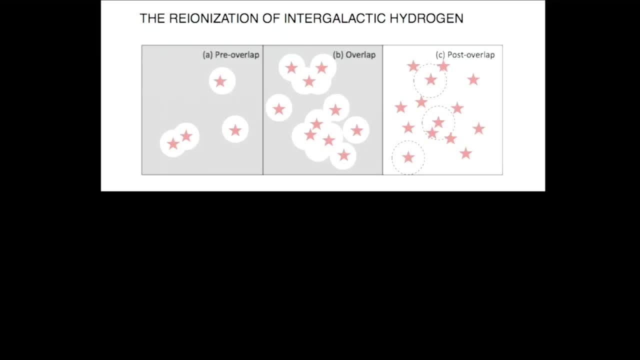 from those galaxies impacted on the surrounding gas and started breaking the hydrogen into constituent electrons and protons, ionizing the hydrogen. So there were these bubbles of ionized hydrogen produced around the locations of the first galaxies And the hydrogen was released into the atmosphere. 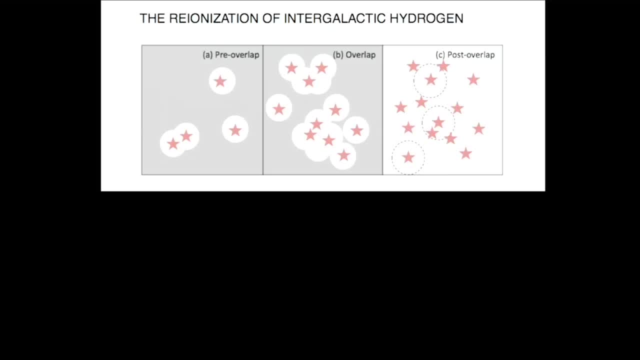 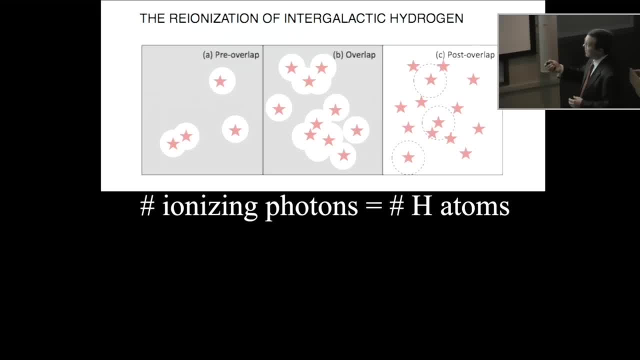 And it's very easy to work out the size of these ionized bubbles as a function of cosmic time. All you need to do is accounting. You just need to compare the number of ionizing photons that were produced and equate it to the number of hydrogen atoms. 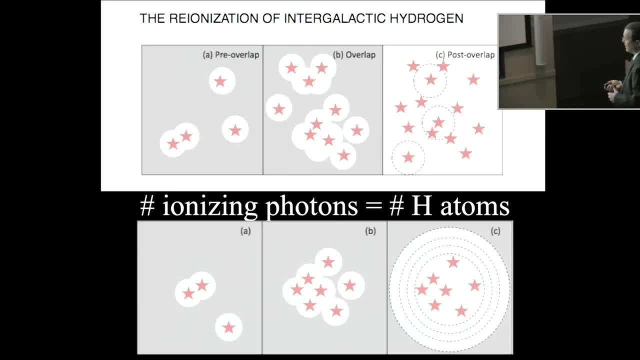 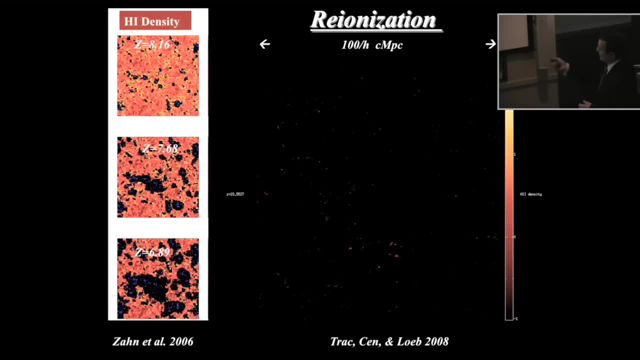 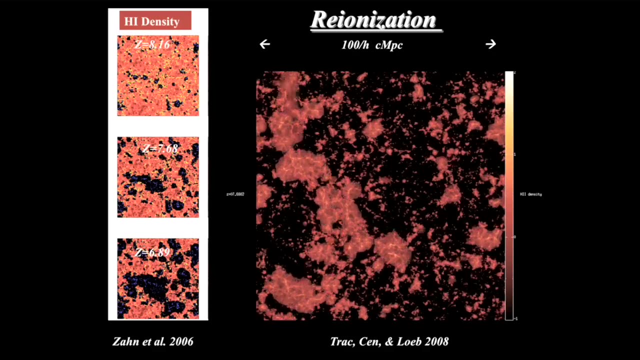 And then you can figure out how these bubbles grow analytically. And here is the result from a computer simulation that takes into account, as a function of cosmic time- so redshift is ticking on the left- how these bubbles grow and eventually overlap. 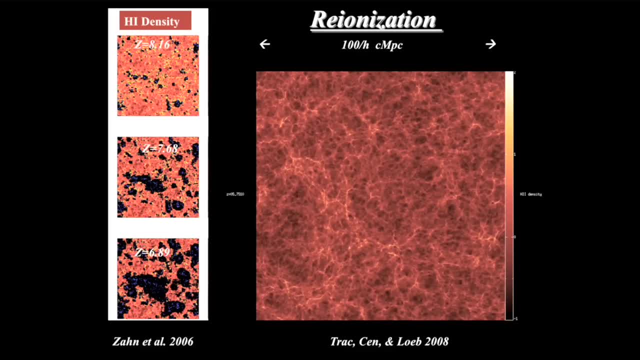 The size of this simulation box is a hundred H inverse co-moving megaparsecs, so it's very big, But as you can see the bubbles towards the end of the process, They are as big as 50 to 100 co-moving megaparsecs, so they really require a very large simulation. 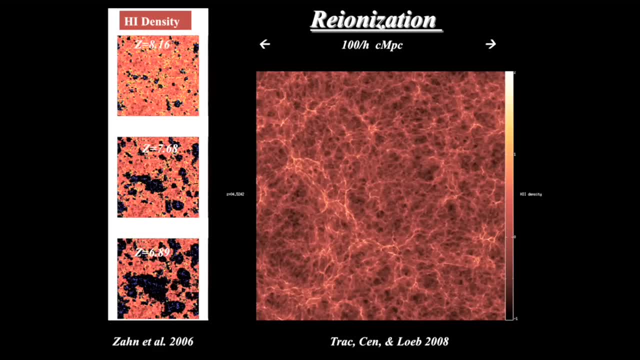 box, and that poses a challenge for numerical simulations, because you need a large box to simulate to get the first sample of the universe. At the same time, you need to resolve very small galaxies that are producing the radiation, So that's why this calculation is very challenging. 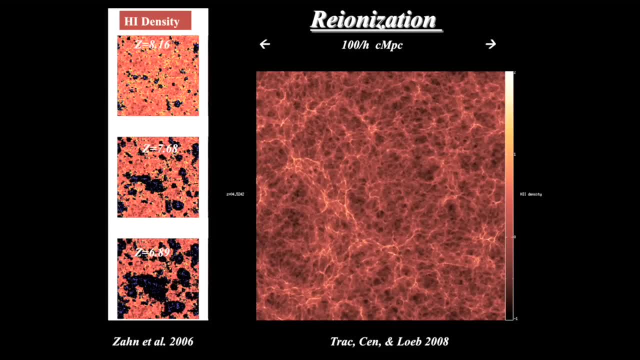 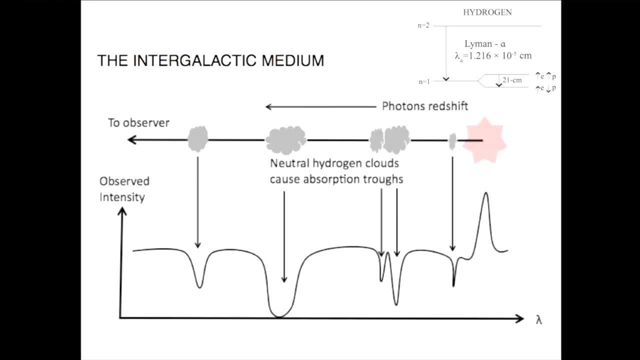 Only right now people are able to make adequate simulations. The traditional method of probing the gas in between the galaxies was using a bright source of light, just like a flashlight, and looking at the interaction of the light with clouds of gas along the line of sight to the source. 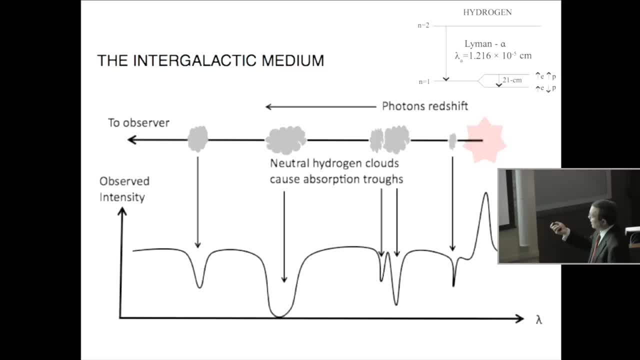 So the type of source that was used very frequently are quasars, bright accretion, black holes at the centers of galaxies, And when observing the spectrum, the rainbow of the quasar, people were able to measure the absorption of hydrogen associated with the concentrations, the regions where hydrogen 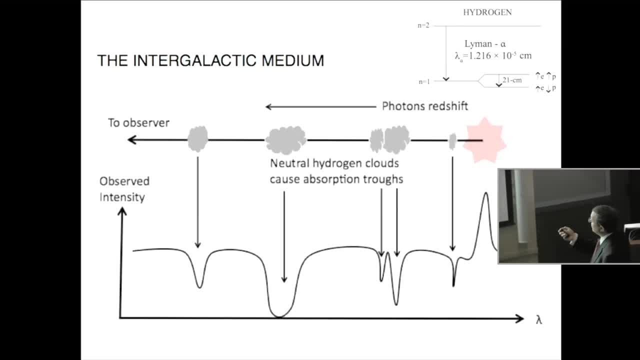 is more abundant And the line that was used is the Lyman-alpha line, the transition from the ground state of hydrogen to the first excited level. So this was the traditional method, Thank you. And the problem of that method is that even trace amounts of hydrogen already produce. 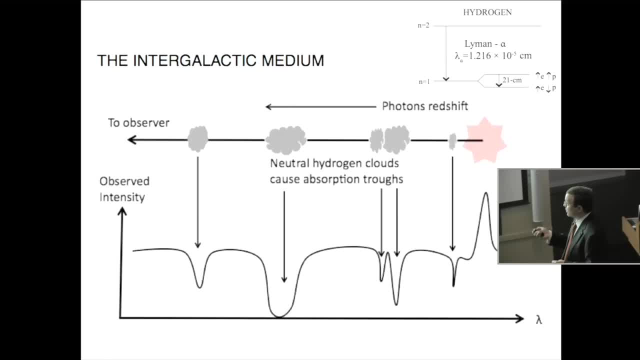 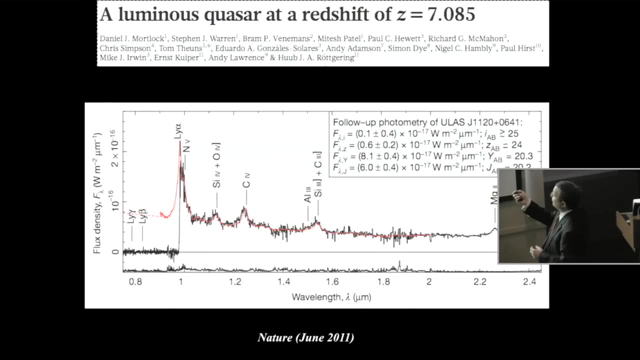 absorption that is almost complete, And so if the universe contains a lot of hydrogen, you can't really see anything because all the flux is being absorbed. So this method is not really effective at probing the process of realization. And you can see that for the highest redshift quasar- at redshift 7.1, there is in the 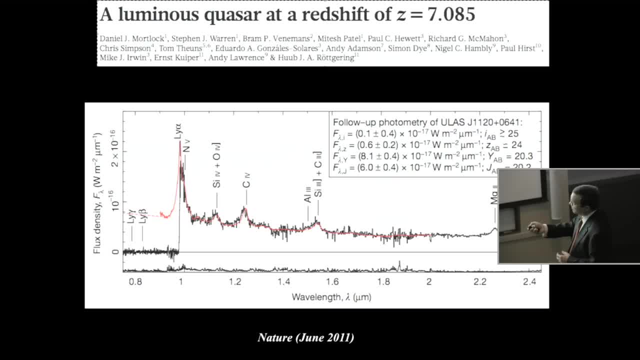 observed spectrum, there is complete absorption. There is total absorption of the flux, short word, of the Lyman-alpha wavelength at the source, redshift, And we can't really tell which fraction of the hydrogen is in the form of atoms back at that time from looking at the flux that was transmitted, because all the flux was 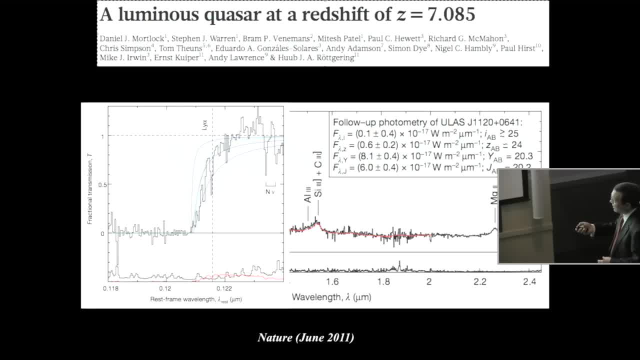 absorbed. However, if you analyze the damping wind of this line, you can compare what you would expect for 10 percent of the gas being neutral, 50 percent or 100 percent. So it looks like back in the day there was no absorption. There was no absorption. If you look at the redshift of 7.1,, a substantial fraction of the gas was already atomic and the process of realization was not complete. But there is a better method of probing the gas using a different transition, and that's. 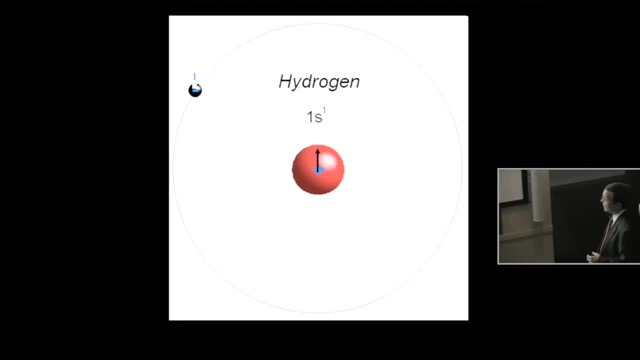 the transition associated with a flip in the spin of the electron relative to the spin of the proton. So in quantum mechanics a particle, an elementary particle, has a spin, as if it's spinning. The spin can be either up or down. 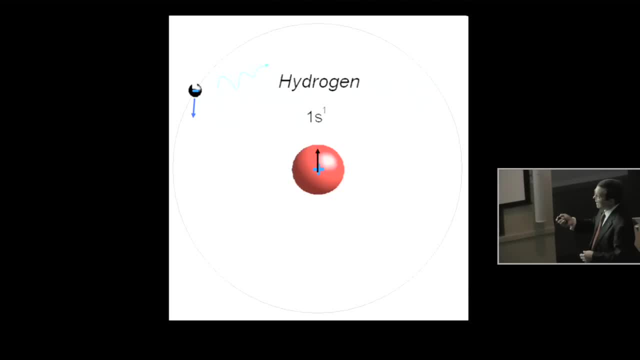 And the spin of the electron can be either aligned or anti-aligned with respect to the spin of the proton in the hydrogen atom, And if the spin of the electron flips, a photon is being emitted with a wavelength of 21 centimeters. So this transition was predicted back around 1940, and there is a connection to Harvard. 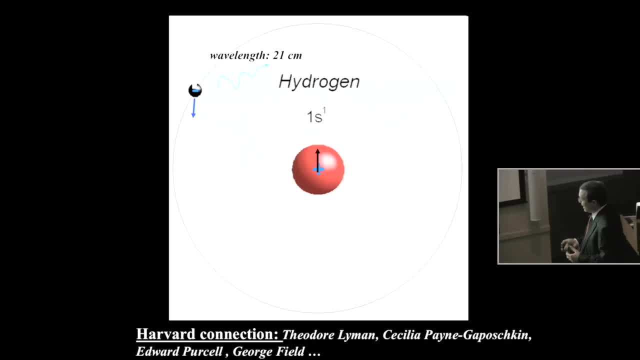 after it was predicted And, of course, hydrogen was realized to be the most abundant constituent. So it's a very interesting transition. It was the constituent of the sun and of the universe by Cecilia Payne-Kaposchkin, But Ed Purcell, once this transition was recognized theoretically, he decided to go out and observe. 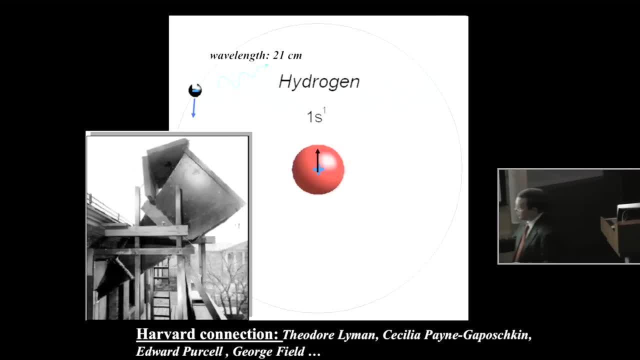 it, And what he did was to open his window, his office window in the physics department, and put a horn antenna through it, And there is still a plaque in the physics building where this horn antenna was placed. The biggest challenge that Ed Purcell faced was that students were throwing snowballs. 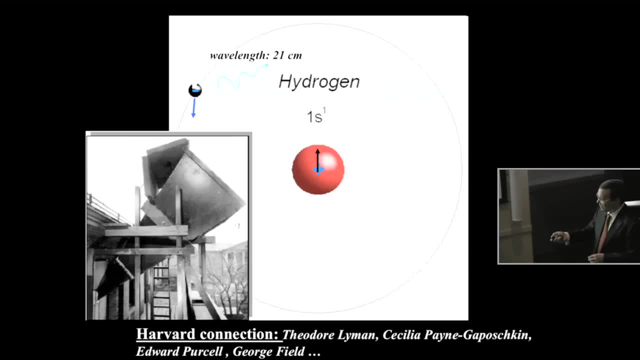 into the horn and they would go all the way to his office. But he managed to get through that and measured very easily the emission from our galaxy. There was a competing experiment in the Netherlands at the time that couldn't get results and Ed actually helped the other experiment. 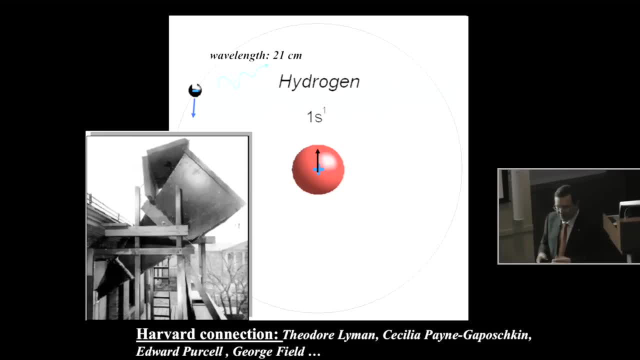 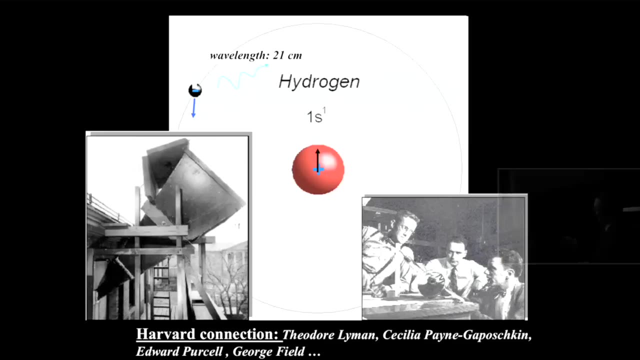 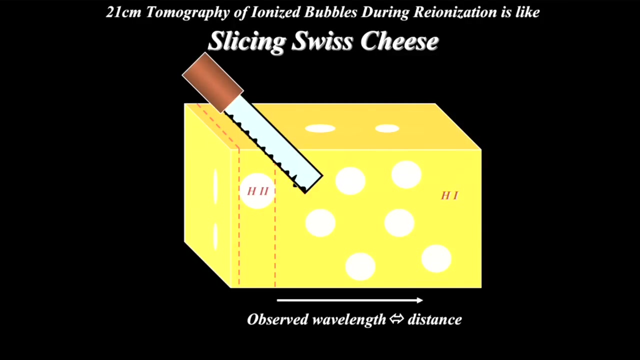 He got the results and published at the same time, So that shows collegiality Back then. I don't think there are many examples that we can mention nowadays for such nice behavior, And this is Ed Purcell. And the idea now in the context of mapping the hydrogen in the early universe is similar. 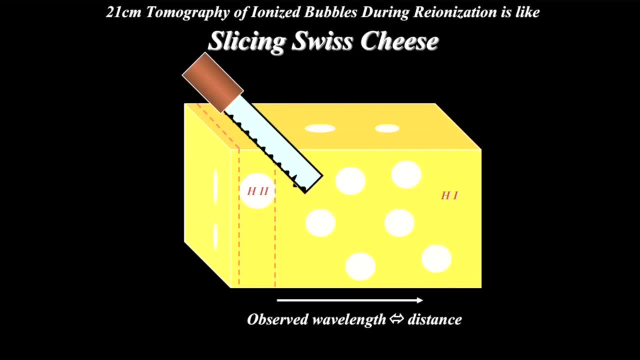 to slicing Swiss cheese. So imagine Swiss cheese that has holes in it. The situation is similar to the hydrogen in the early universe that had holes or ionized regions around groups of galaxies, And what we would like is to slice space just like slicing Swiss cheese. 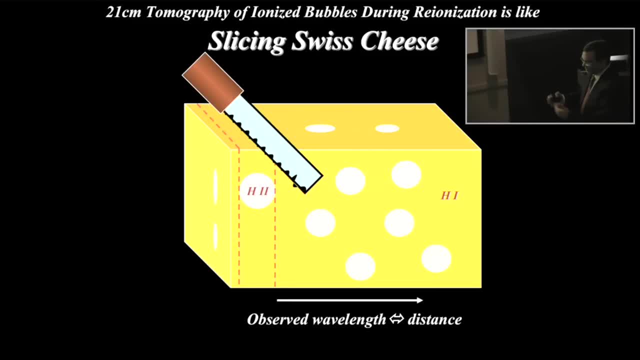 And we can do that because the observed wavelength, the wavelength that we observe on Earth, is being redshifted by the cosmic expansion. So, as we look at earlier times, there is more redshift that this wavelength is experiencing, And so, by observing different wavelengths, we are able to slice the universe at different. 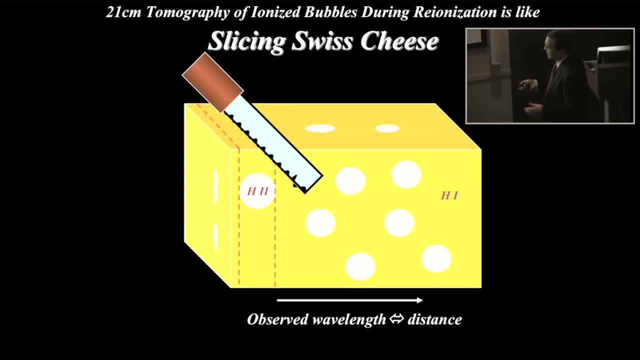 redshifts, And we can slice it in principle also in three dimensions, because we have the two dimensions of the sky and then the dimension of redshift along the line of sight into the universe, And this is what theoretically we would expect. 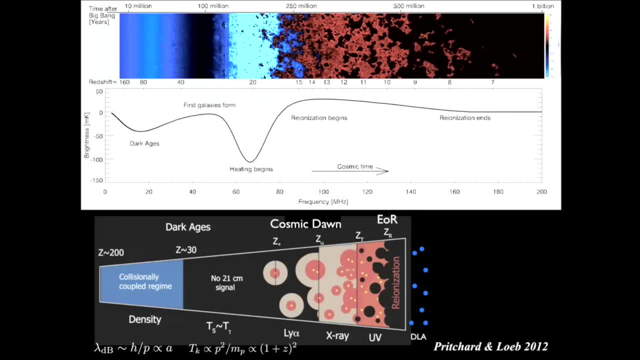 That's an image of the hydrogen that was produced by theorists. We hope to see it in the real sky over the next decade, And what you see here is a two-dimensional illustration. So there is one dimension on the sky and then another dimension of depth into the universe. 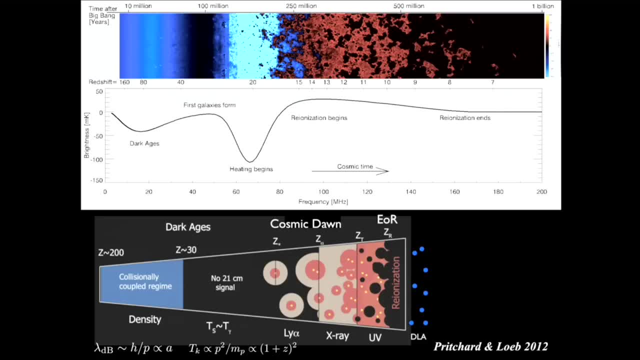 And what we're looking at are different times in the evolution of the universe. So that's 10 million years after the Big Bang, 100 million years after the Big Bang, 200,000 years after the Big Bang, 250 million years, 500 million years and the corresponding redshifts to those times. 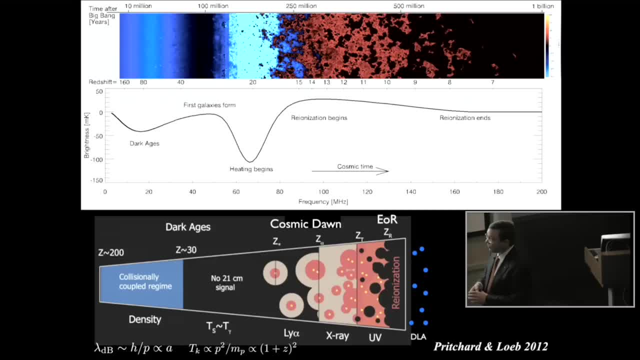 And blue indicates absorption of the cosmic microwave background by the hydrogen. So the brightness temperature is negative at very early times because the gas at redshifts below 200, the gas was cooler than the microwave background so it absorbed at the 21 centimeter. 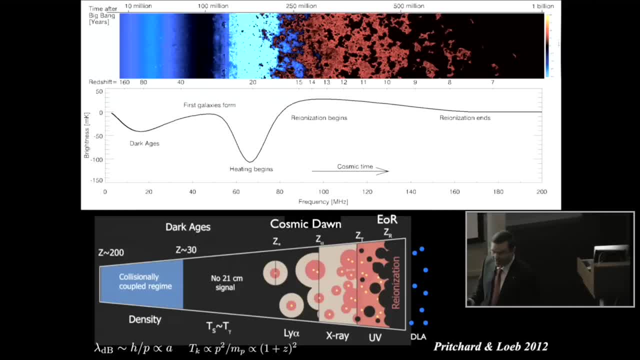 transition. The universe was relatively smooth because there were no galaxies formed at that time. Then, at some point, the coupling- the radiative coupling of the excitation temperature of hydrogen to the microwave background was more important than the collisional excitation of the gas. 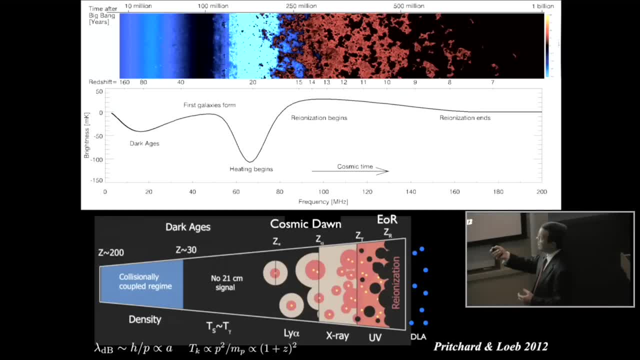 And at that point you couldn't see the gas. It became black relative to the microwave background. That's when the brightness temperature was zero relative to the microwave background And then the first galaxies formed around that time, A hundred million years after the Big Bang, they produced ultraviolet radiation that allowed 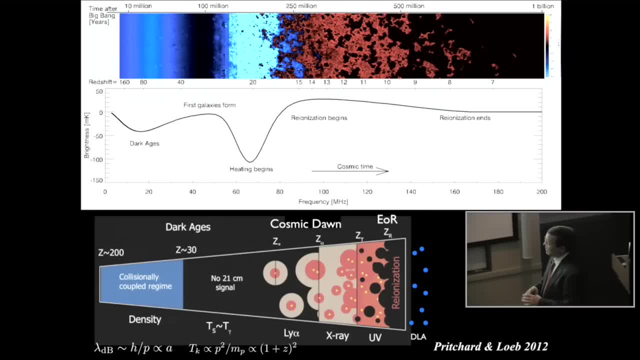 the excitation temperature of the gas to couple once again to the kinetic temperature of the gas, making it again appear in absorption Around. that time you start seeing those smudges due to the localized emission from galaxies And then also X-rays that were produced by the first galaxies heated the gas so that 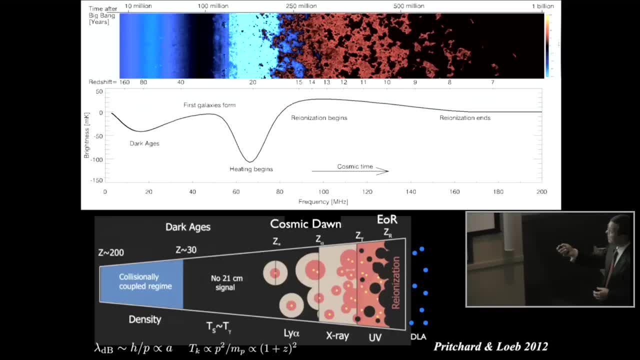 eventually it started to appear in emission. So that's what happened And that's in red here. So more than 250 million years after the Big Bang, that's when the gas started to appear in emission, and emission dominated the picture. You see, everything appears in red at later times. 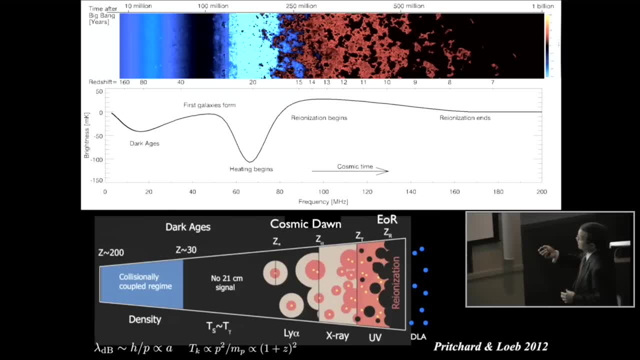 But there are all these holes, the holes in the Swiss cheese that were produced by groups of galaxies And eventually, these black regions where hydrogen does not exist because it was ionized, overlapped, at redshifts below six and a half or so. 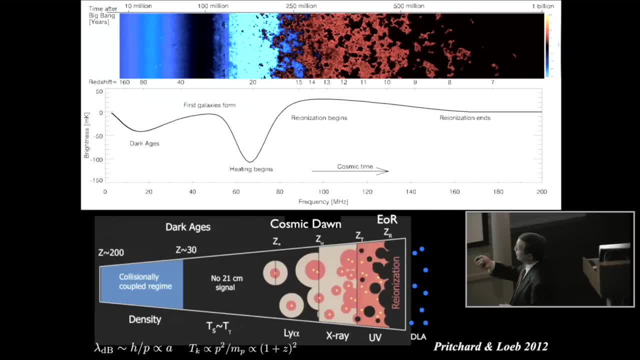 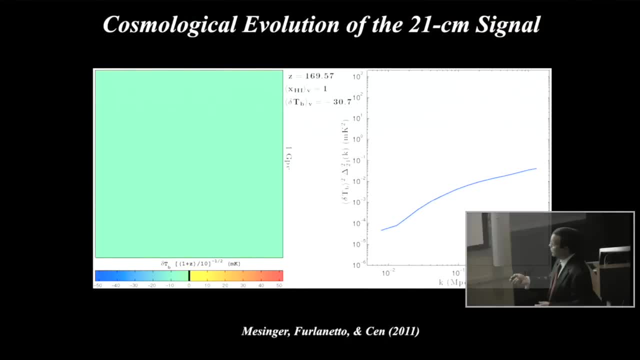 And there is no hydrogen left for us to see. So this is the theorist view of what the observers should find over the next decade, And that's a simulation result of the same picture that I described. You can see the redshift ticking here at the top. 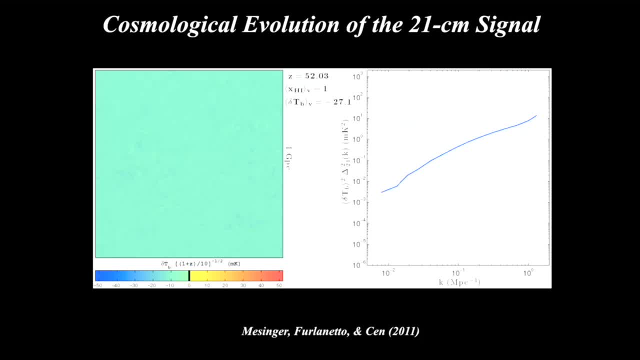 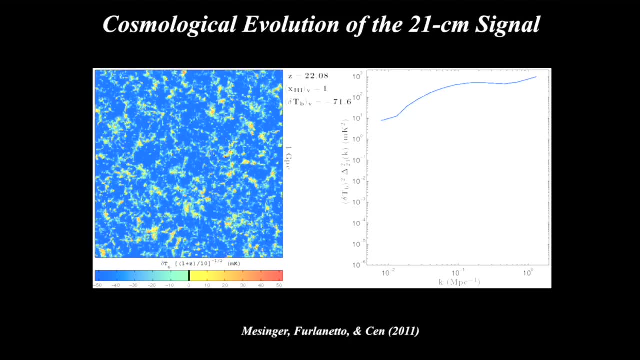 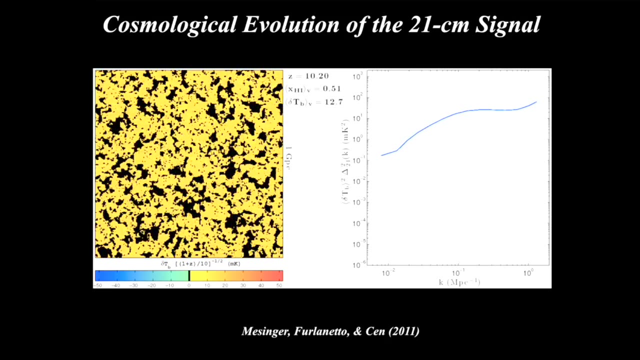 And as time goes on, as the redshift goes down, the signal in the brightness, temperature fluctuations of the gas, the hydrogen gas, changes. So this is the power spectrum of the 21 centimeter fluctuations And you see here that as we go to redshifts below 10 or so, that's when the ionized bubbles start to grow And eventually they overlap by a redshift of seven or so. And there are a number of experiments aimed at measuring those images that we theorists predict. There is the low-frequency array. There is the low-frequency array. There is the low-frequency array. 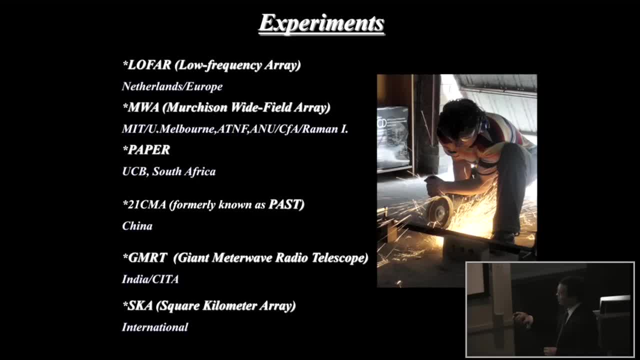 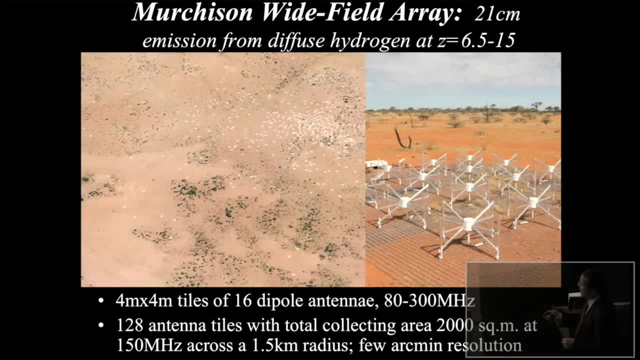 And this is how the pile of dipole and dipole are divided. The dipole of tipole antenna looks like. for the NWA that we are members of, that is an artist illustration of what the final array should look like, And there would be 128 tiles, each of which having 16 dipole antennae. 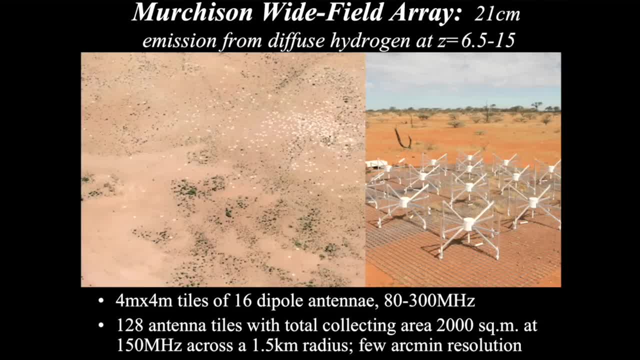 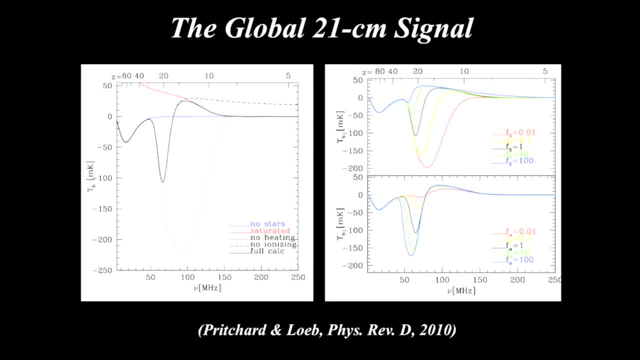 The same size as the old TV antennae that were used through for reception of TV signals back in the 60s principle. you can also average over the sky and measure the spectrum of the sky, and that's called the global 21-centimeter signal, which will be. 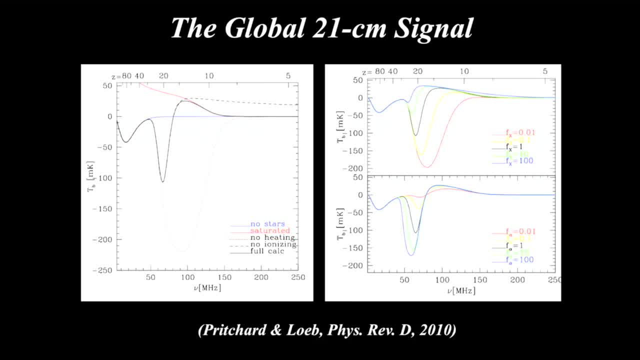 sensitive to how much X-ray heating was produced. So if there was no heating whatsoever, that's the dotted line. there is a very deep absorption trough in this spectrum of the sky. You can imagine also having no stars whatsoever, where the signal would look like the blue line here. So the 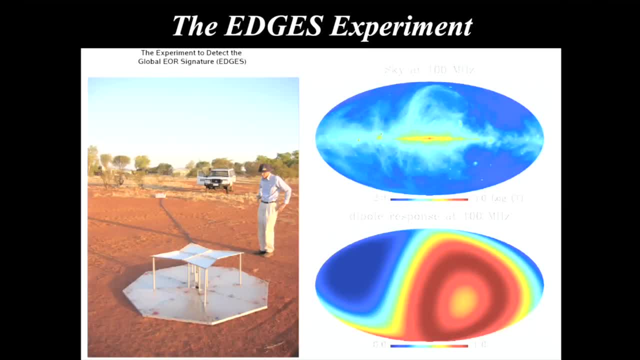 details of the signal tell us something about the first generation of stars, And the interesting thing is that this global signal can also be picked up by a relatively modest single antenna, and this is an experiment led by Alan Rogers and Judd Bauman that I'm always proud of describing because it 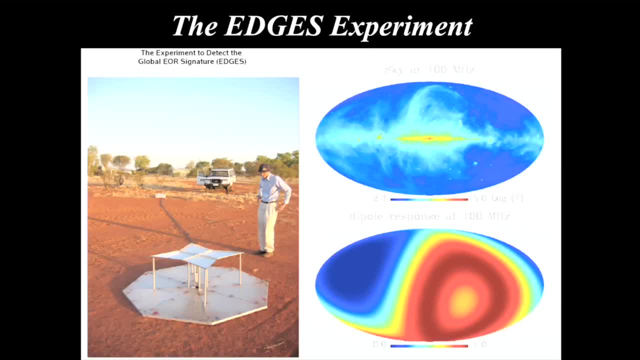 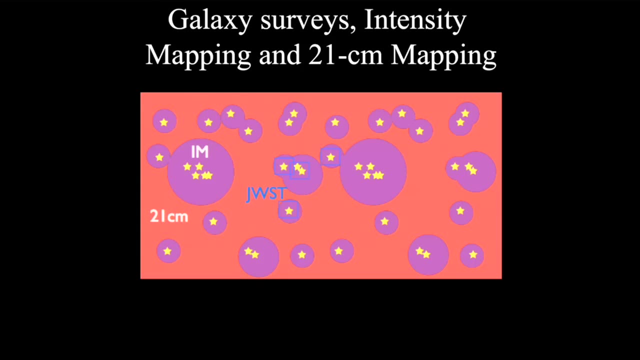 shows that two people with a relatively modest budget and good ideas can actually advance the frontier of science. You don't need big groups necessarily, you can think independently. And finally, one can use other lines other than the 21-centimeter line of hydrogen. So the 21-centimeter line maps the hydrogen outside of the regions. 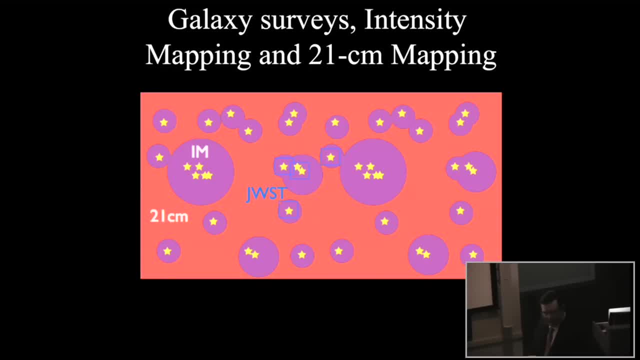 where you find galaxies, but you can imagine the galaxies themselves emitting spectral lines and one can map those, this emission, without resolving individual galaxies. So that's very different from a galaxy survey. You're not trying to resolve individual galaxies, you're just looking at. 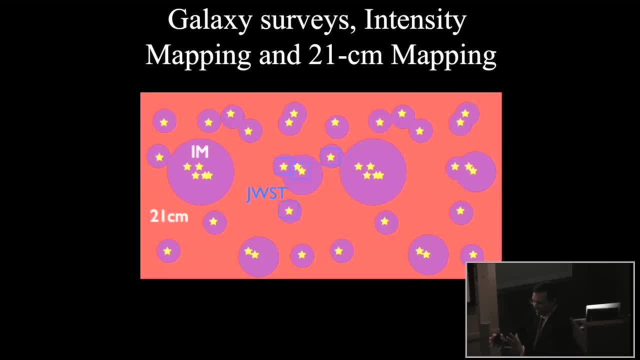 the cumulative emission from groups of galaxies. There are more galaxies in particular regions of the sky. therefore you would get more intensity in those spectral lines. and you can do exactly the same as the 21-centimeter method. You can map in three dimensions the distribution of galaxies. in this case, 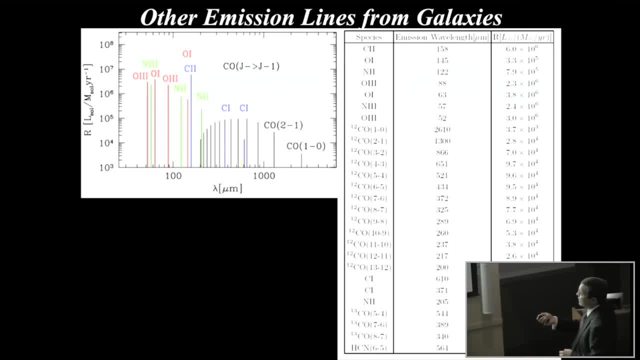 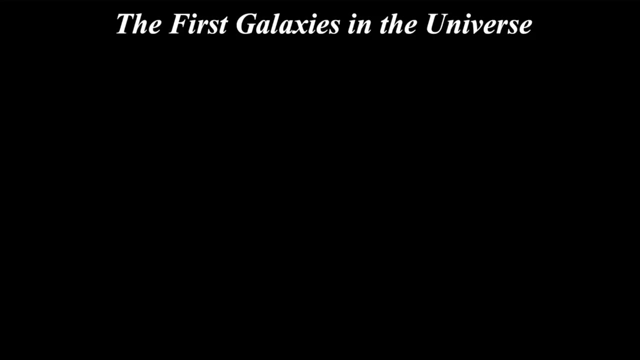 or matter, and there are many different lines that one can use at the millimeter or sub-millimeter wavelengths. that would be of course redshifted to some centimeter wavelengths, And so let me summarize. I gave you sort of a sketch of 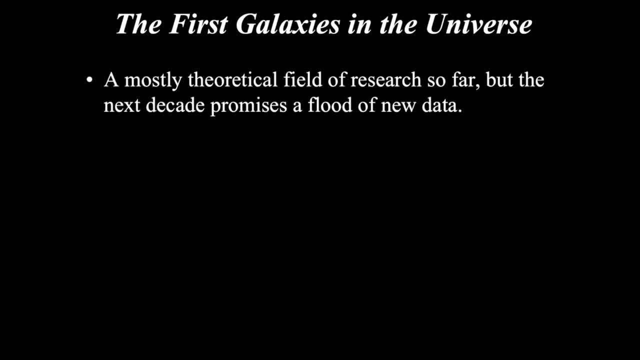 the various interesting frontiers in this context. This was a mostly theoretical field of research so far, and that's why we decided to summarize it in this book, but the next decade promises a flood of data, and the prediction that I can make that is that if the second edition of the book will look similar, 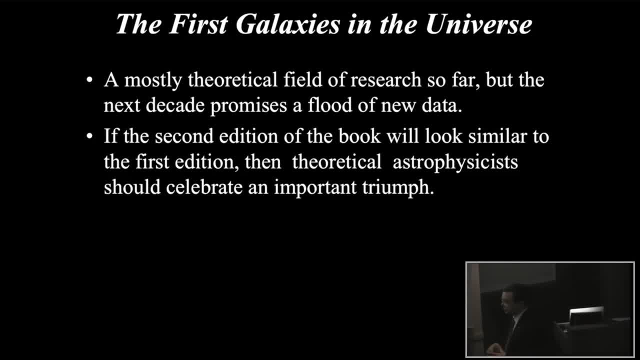 to the first edition, then theoretical astrophysicists should celebrate an important triumph, because we were able to predict, to forecast what the observers would see. But we should not assume that the data will show agreement, and so, if not, of course I will have to rewrite some parts of this book, and that's. 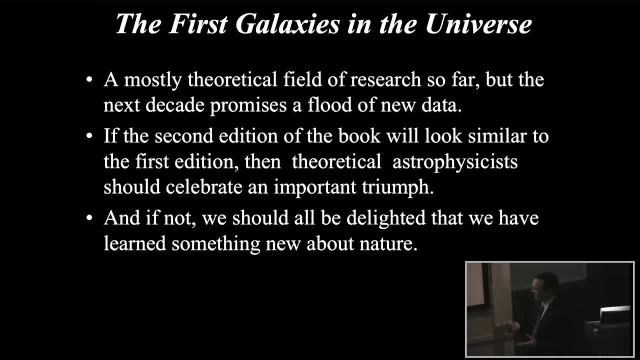 unfortunate, but we should also be delighted that we learned something new, and the important element of advancing science is that sometimes you should accept that you made a mistake, that you're wrong, that some ideas that you had are incorrect and those areas of science where you don't see people admitting that they made. 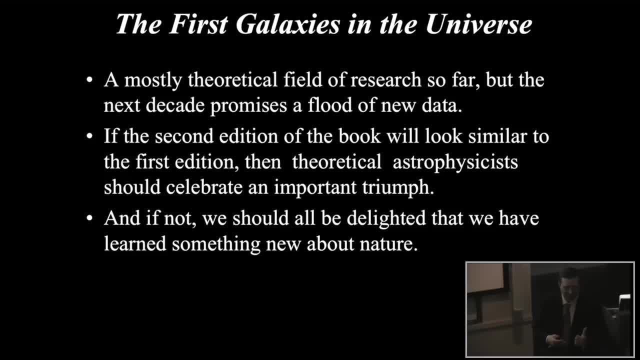 mistakes are those that either have no data or like string theory, or areas where people are simply not making predictions. So if it's a very healthy element of science to make progress or improve our understanding based on data that falsifies existing notions- and we would- 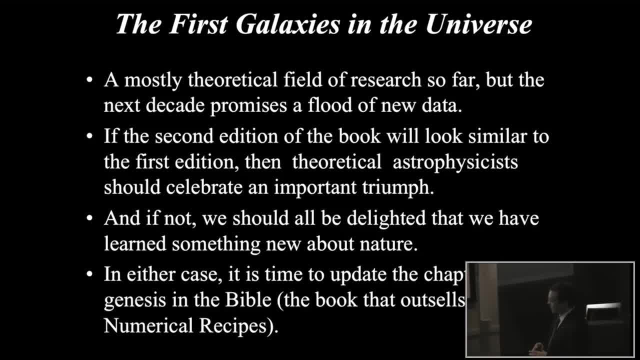 be, of course, delighted if we learned something new, But in either case, I think it is time to update the first chapter of the Bible and if anyone wants to know what any of those secular people in the audience, that's the book that sells more. 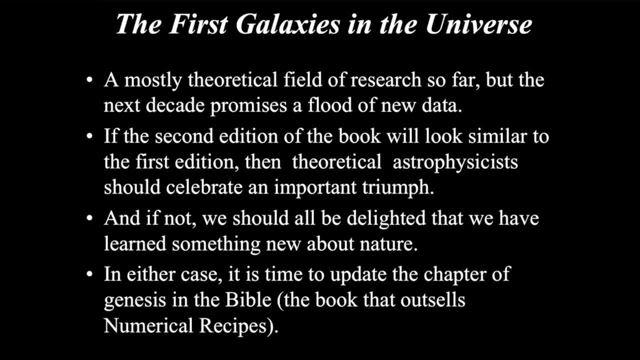 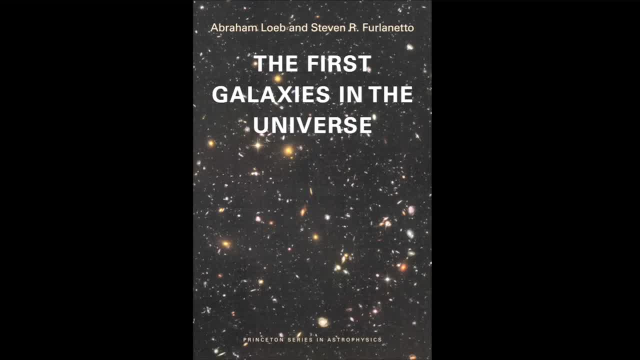 than numerical recipes. Thank you, I'll take a few questions if you'd like to ask. Can we pull the lights up a little bit in the back there? Thank you, Questions. I think it's time for refreshments, Rick. So I understand that the plot causing the background radiation data is very, very very. 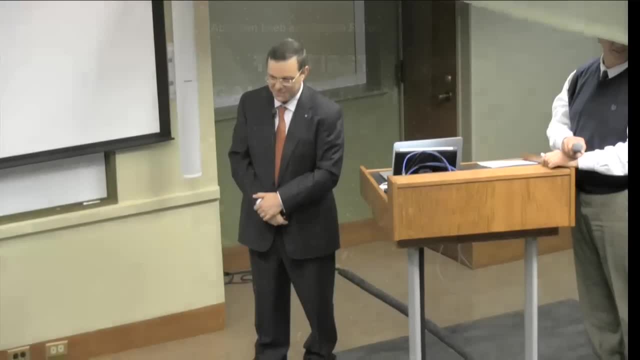 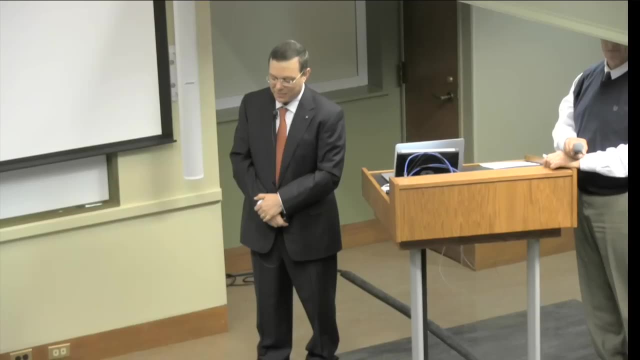 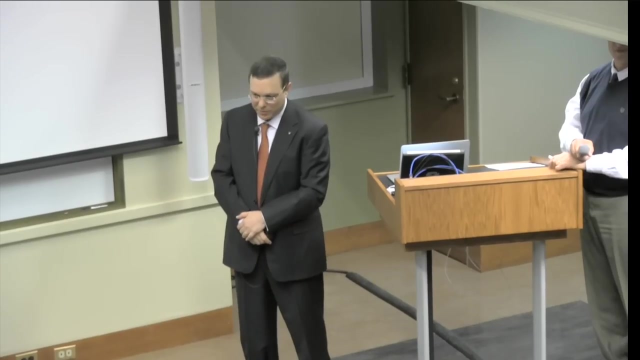 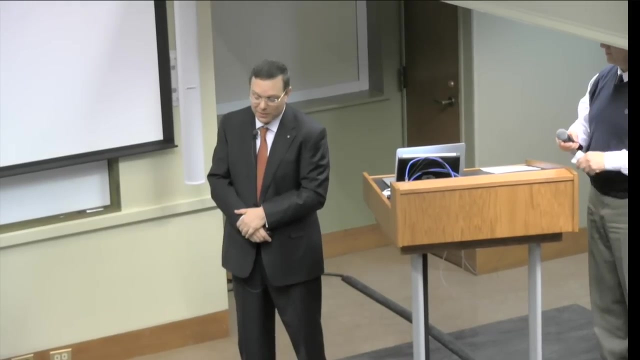 complex. Yeah, Yeah, That's right. What are you anticipating to learn from that as it applies to the scenario? Well, the plot data is much more detailed than the WMAP data that we had before, So it will most likely give us better, tighter error graphs, But it could in principle. 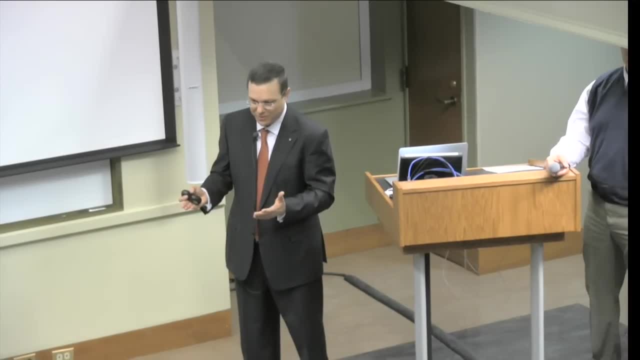 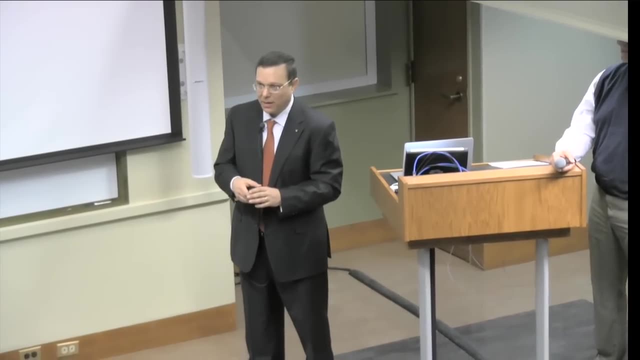 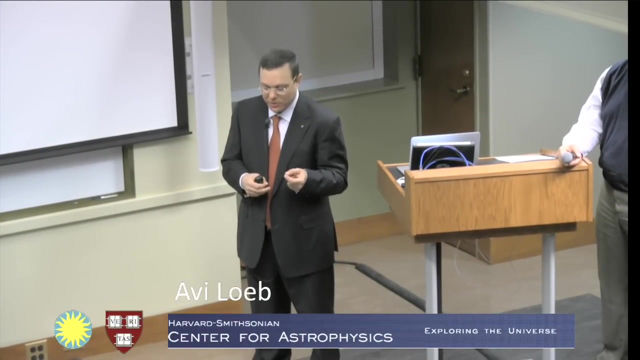 reveal the existence of another neutrino species, or could tell us that the power spectrum of the primordial density fluctuations was not a pure arrow, for example. There could be surprises in this data, just because of the precision. that gets better, And so that will. 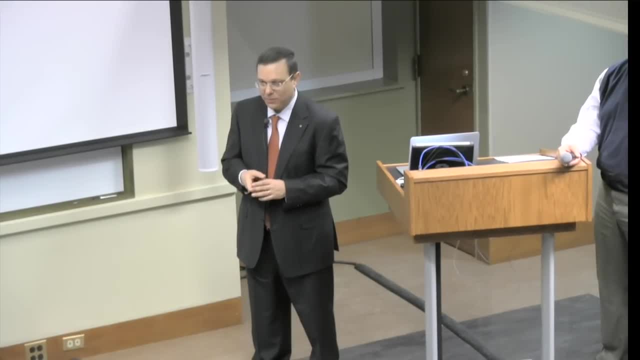 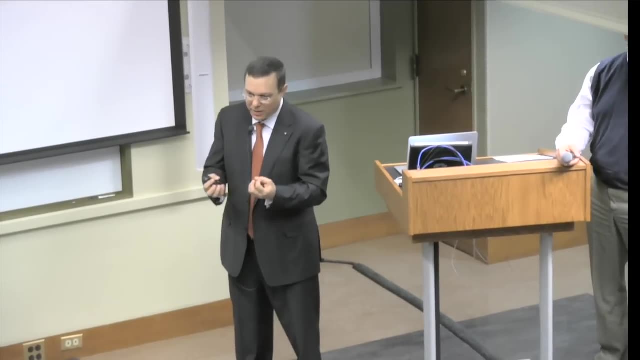 of course have implications for the first objects, because we are dealing with a structure in the universe formed hierarchically. The first objects were smaller and they later ascended to make bigger and bigger hellos And therefore the predictions that we make. 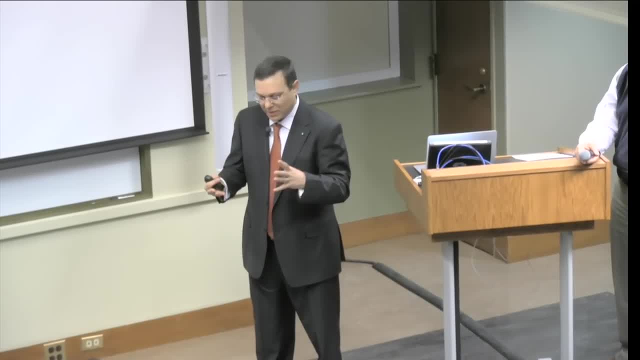 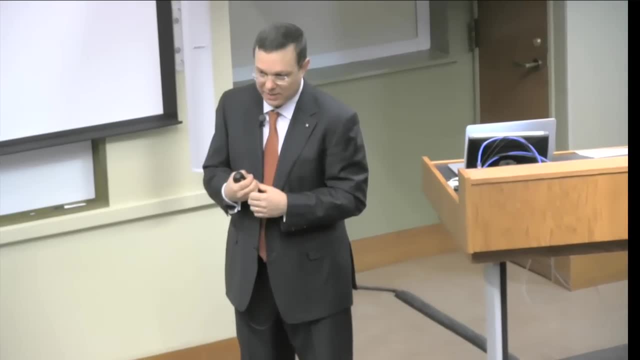 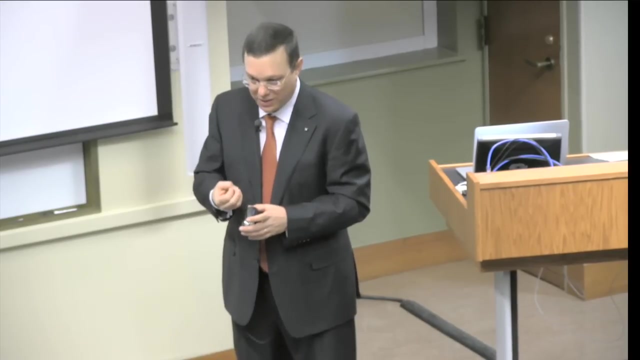 depend on the amplitude, the level of inhomogeneities in the universe on very small scales at early times. We haven't probed these scales yet And that's of course the reason why we want to go to early times to see the initial conditions of small scales. But perhaps that 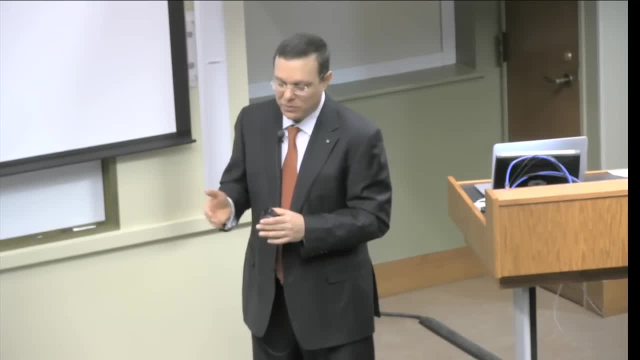 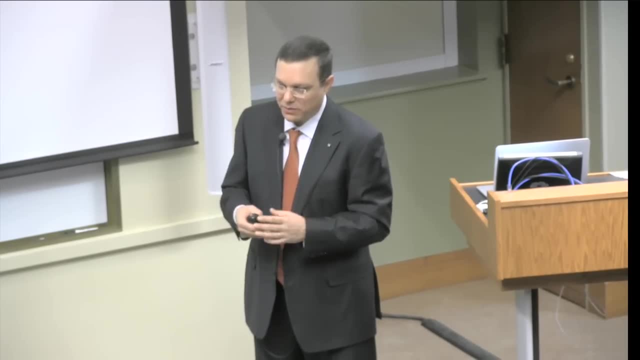 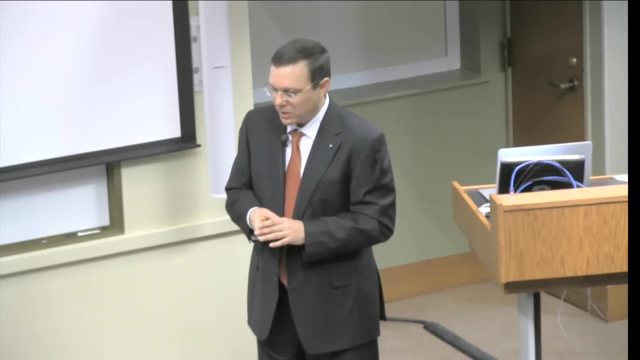 will give us a hint that the power spectrum is not a pure power law, And then we have to correct the predictions for small scales. Any modifications of the standard model of cosmology would be quite exciting, And right now the situation as far as I'm concerned is quite depressing because there is a standard. 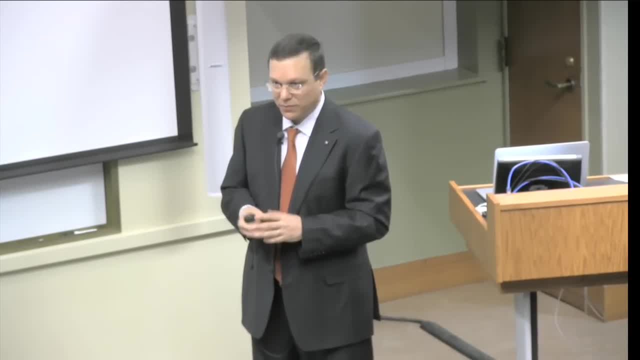 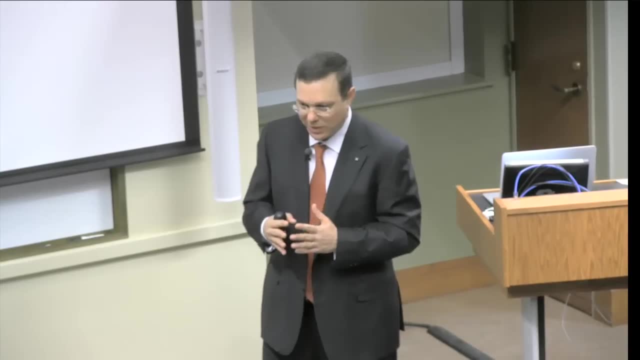 model of cosmology and at least there is a very strong mainstream in cosmology And young people are drawn to be very orthodox with respect to this mainstream view. So I often see young people in our corridor here. that you know. they have a very strong view. 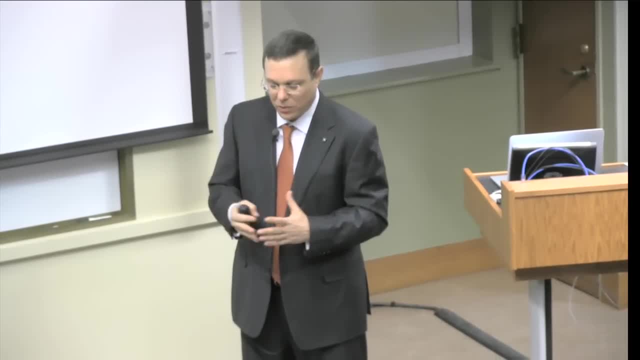 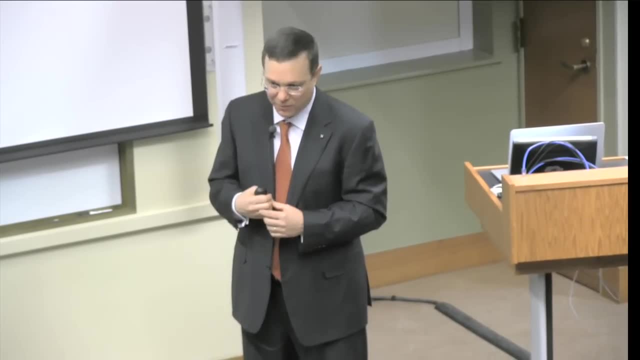 that they very strongly believe and assume that the whole dark matter, the standard cosmology, must be right, that we have the correct notion of the dark matter being weakly interacting with massive particles, with nothing else accounting for the dark matter. And I find 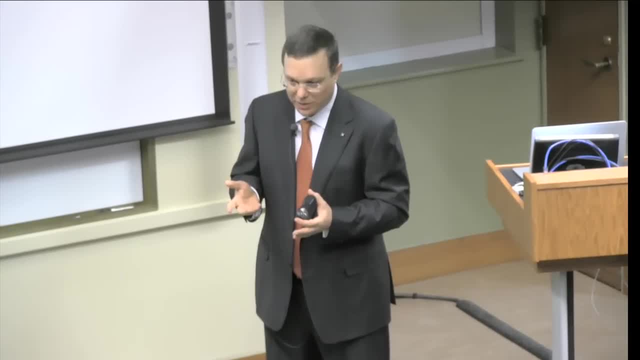 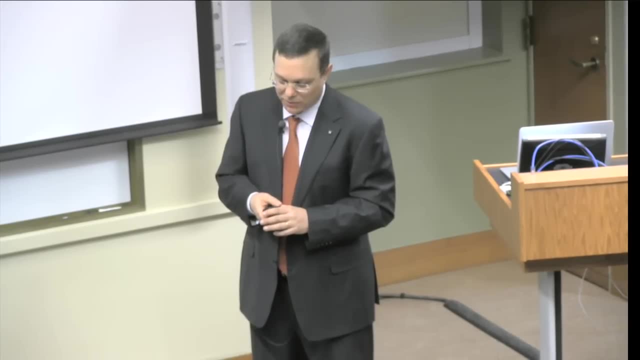